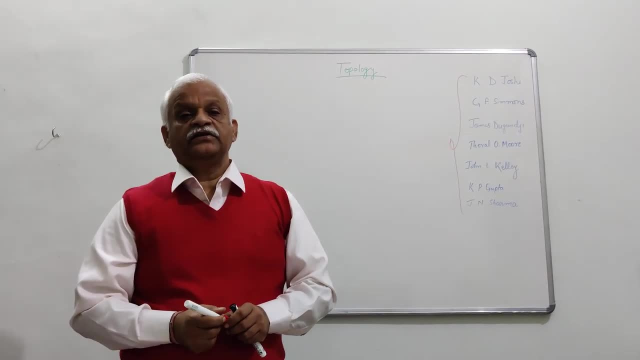 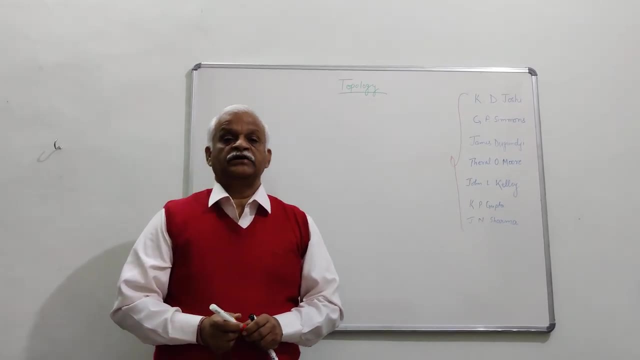 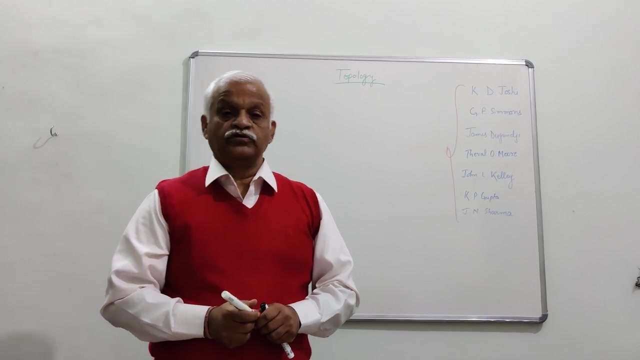 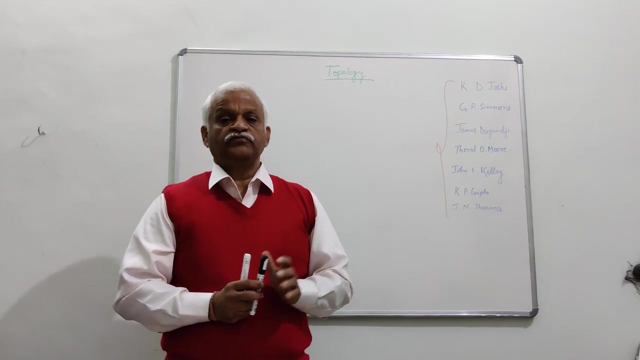 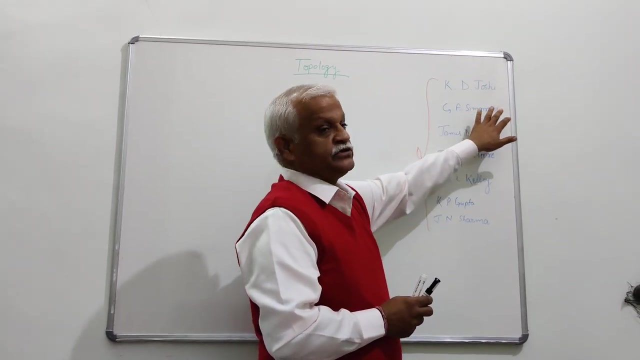 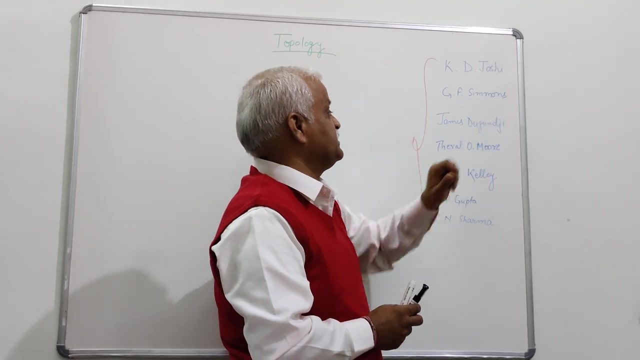 Students, today we will start the second paper of your course, Topology, which is the second paper in semester 1.. First of all, I will tell you about the books, Books I recommend so that you can understand the subject. The best book which I know is by KD Joshi. It is General Topology by KD Joshi, or Introduction to Topology and Modern Analysis, by GF Seamans. 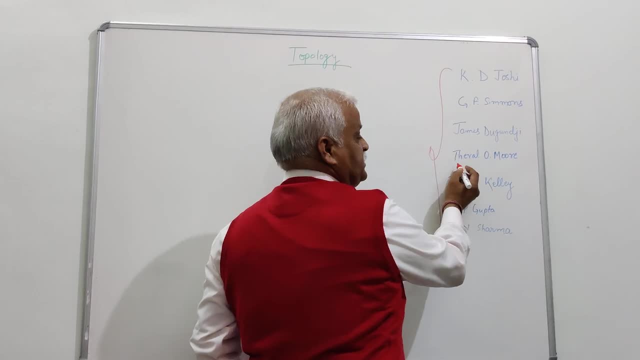 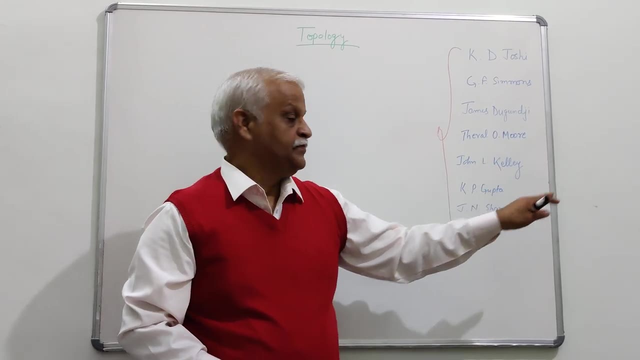 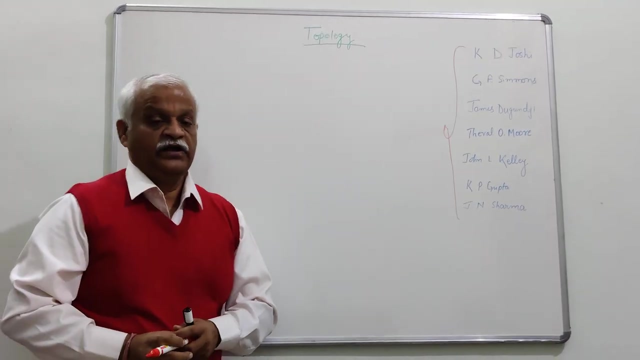 Topology by James Jodungye, Topology by TO Morey or Topology General Topology by JL Kenney. Also, you have books. You have books from Dr KP Gupta and JN Sharma. 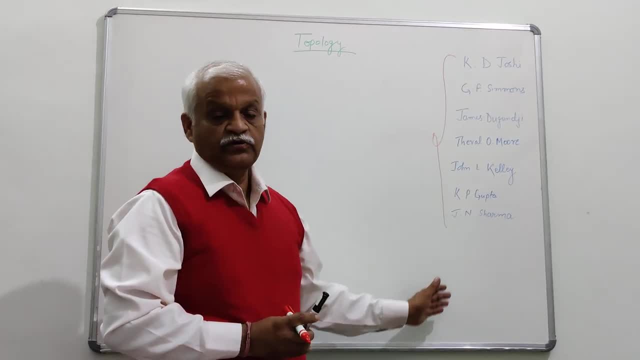 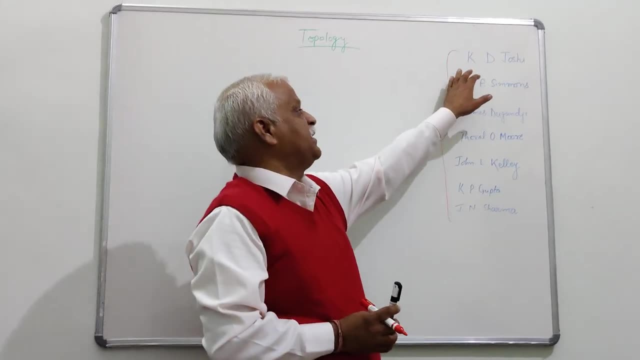 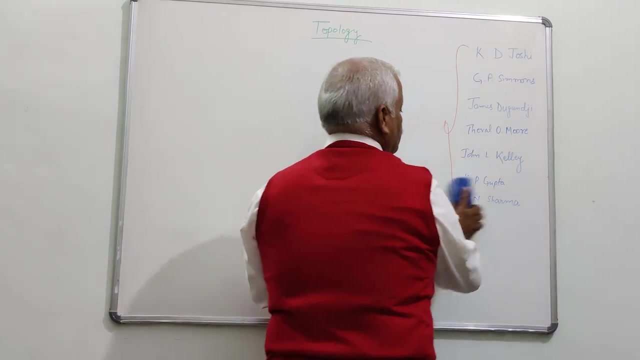 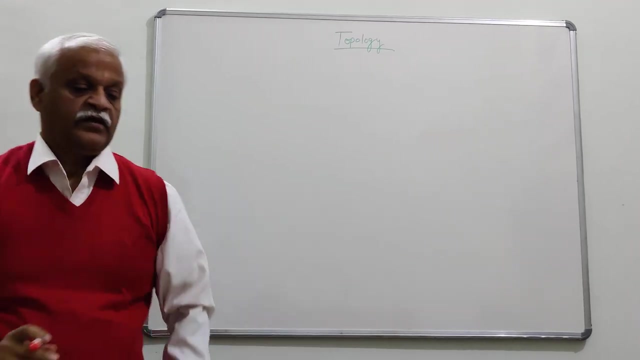 You can purchase any one of these books to understand the subject or understand the concept and examples of the related topics, But I think the best book is of Professor KD Joshi. So we will start. the subject Mathematics can be divided into two categories, mainly. 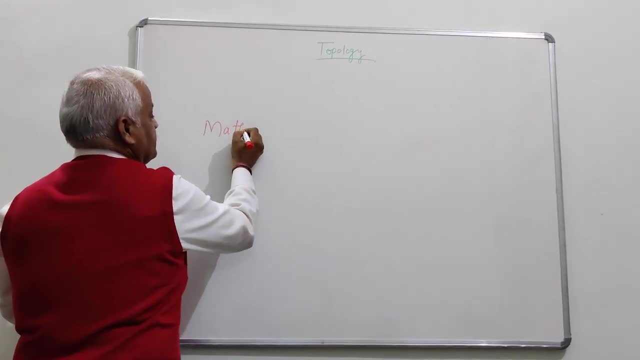 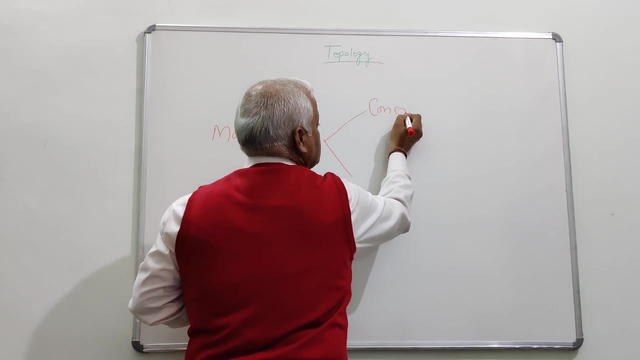 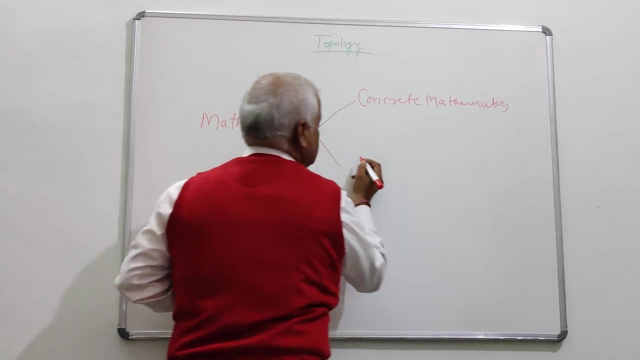 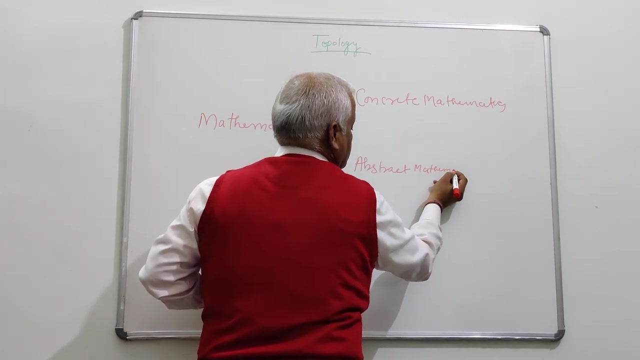 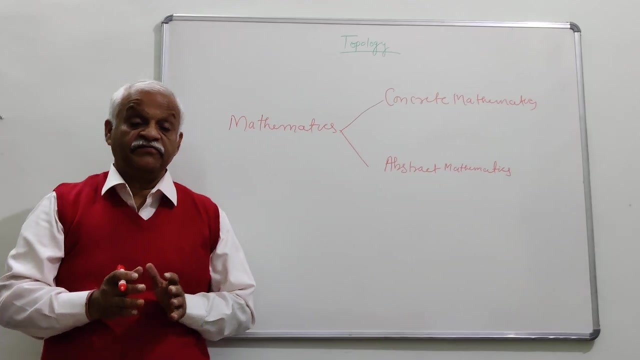 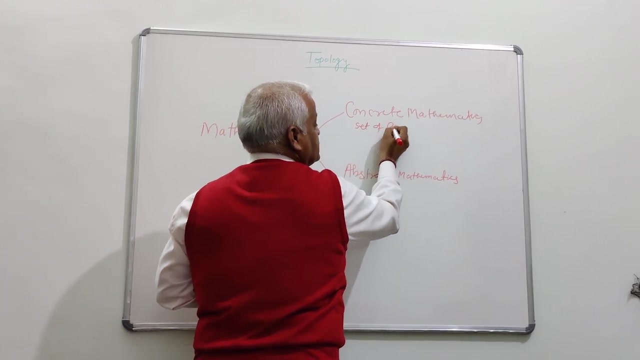 Mathematics is. this is mathematics We can divide in two categories. One is concrete mathematics and other is abstract mathematics. What we do In concrete mathematics we deal with some very specific sets like set of complex number, set of real numbers, set of reals or complex. 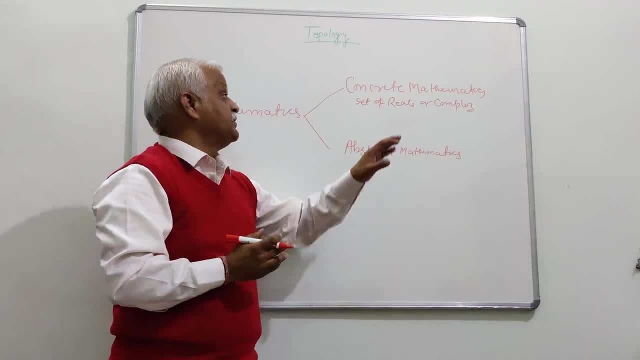 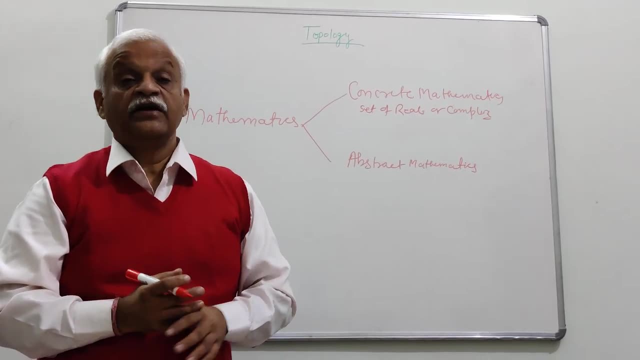 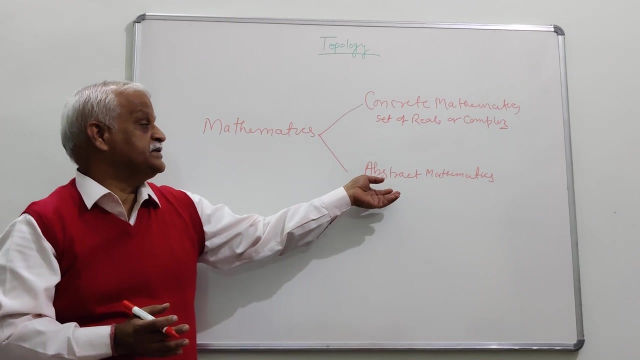 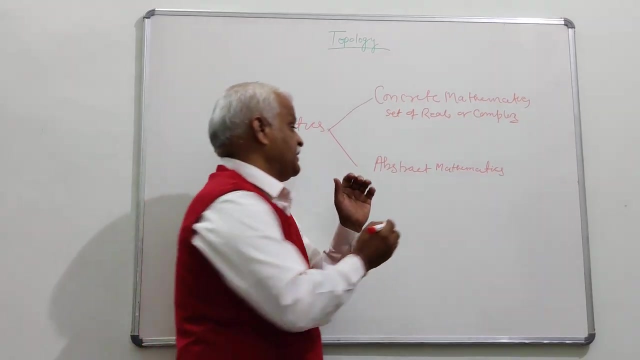 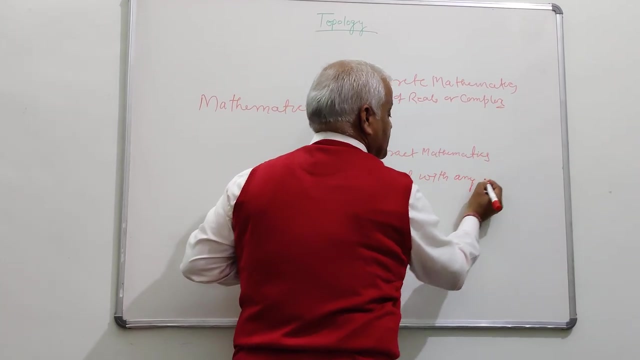 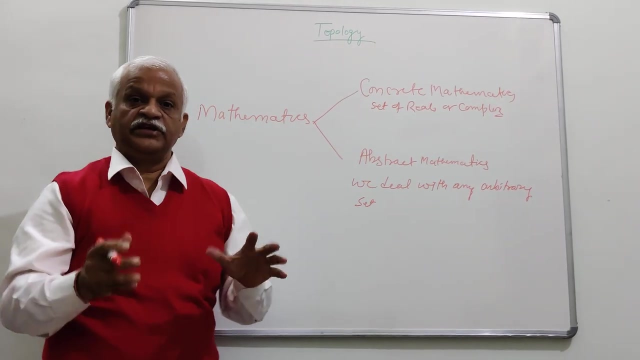 Here the sets are specific From this concrete mathematics. you have already completed the courses of real analysis, complex analysis. they are included in this section. and what happened in second? second is the abstract mathematics. in abstract mathematics we deal with any arbitrary set. we deal with any arbitrary set and put some structure on it. 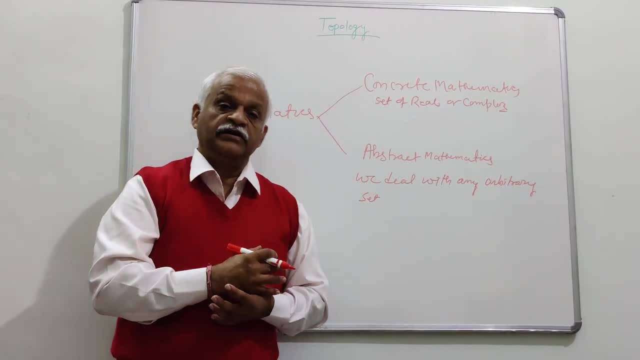 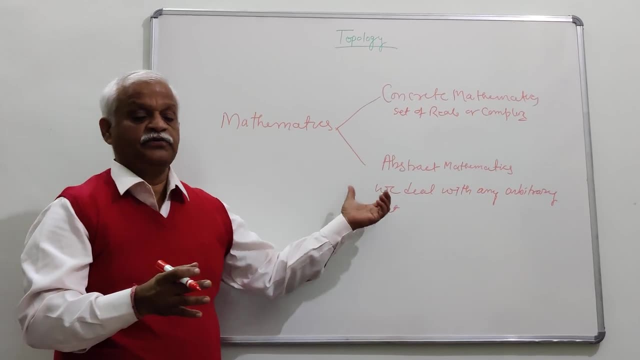 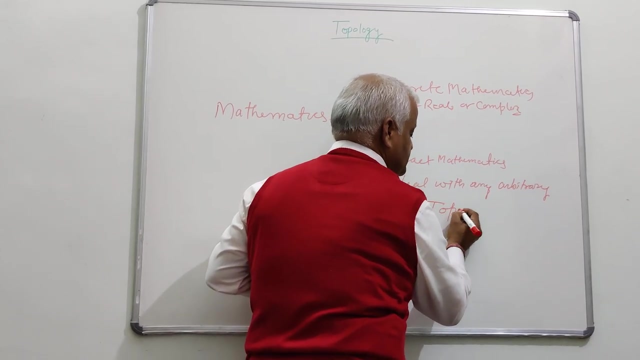 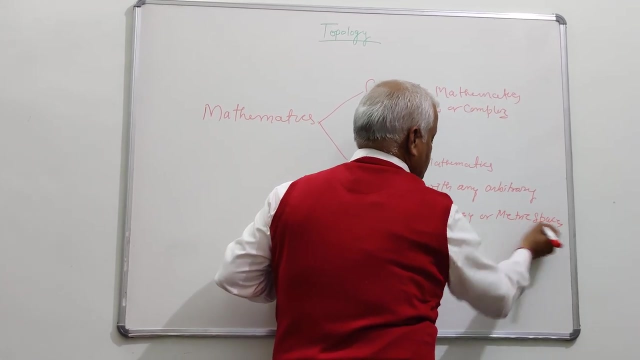 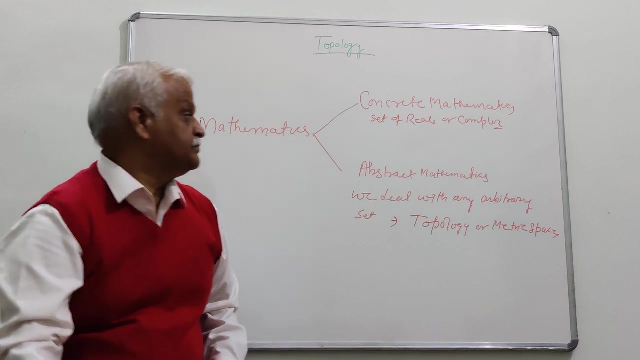 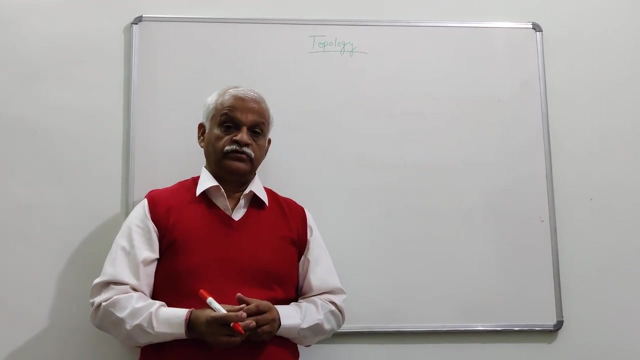 some additional structure. you must know about the additional structure: some binary operation, some function and all that, some additional structure put on them. then we study: and algebra, abstract algebra, topology, matrix space, matrix spaces, topological topology and matrix spaces, like in this category of the mathematics we have to from here this topology arises. you know about the graph theory also. we 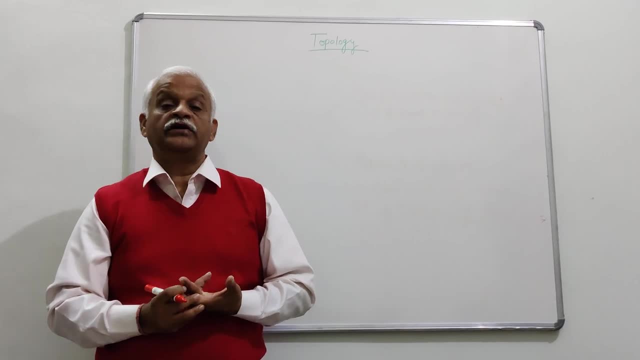 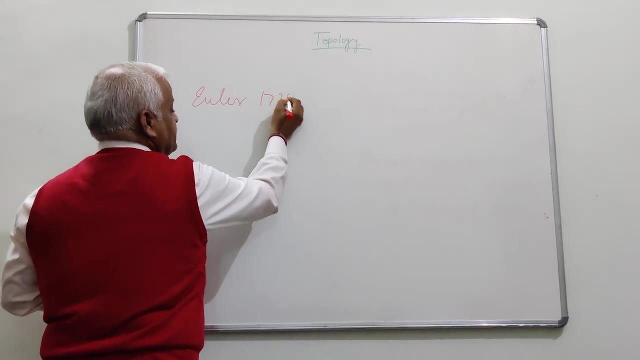 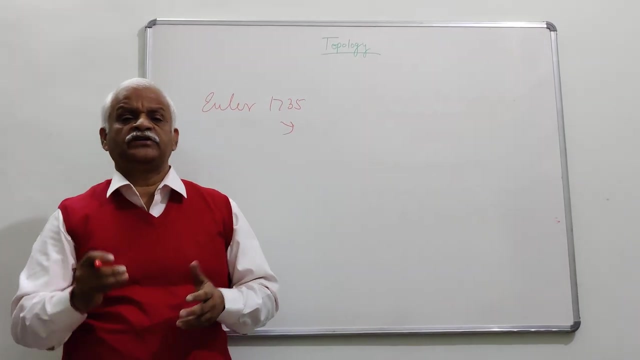 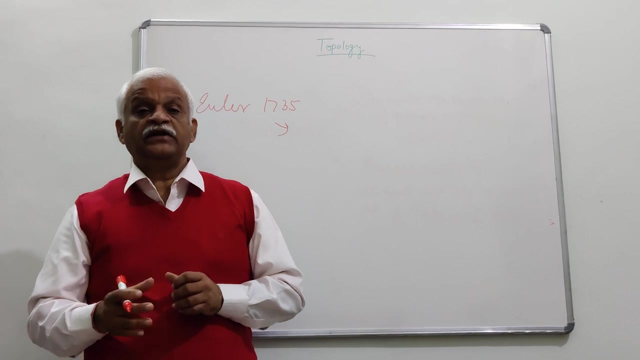 have one problem given by the Euler in 1735. Euler gives one problem in 1735, Konigsberg, seven bridges problem. this is the famous. you can put this on Google, you get it: seven bridges problem. now the name is chain. we have seven bridges on a river and 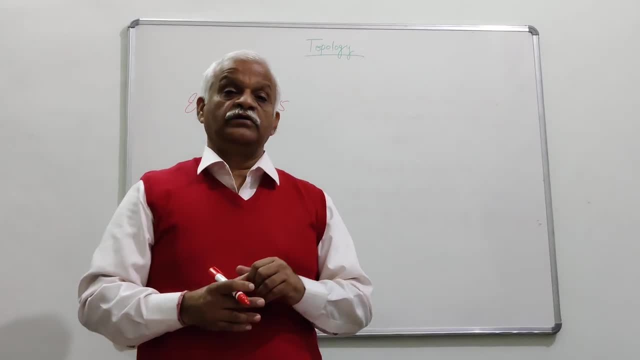 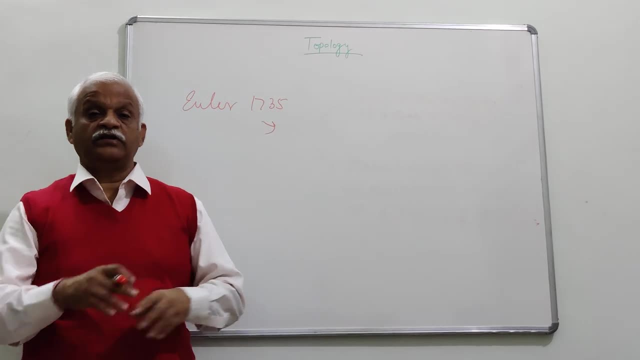 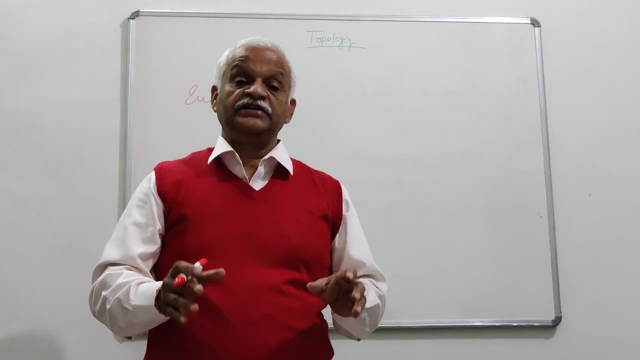 without crossing the bridge, one bridge two times. you have to cross all the seven bridges. and this problem is related not with the geometry, not with the distance. it is related to the connectivity from the connectivity of bridge, from the connection. so now we are going to see how it is related to the connectivity of the bridge. 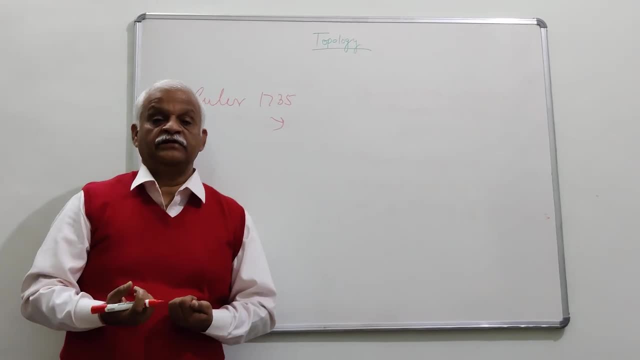 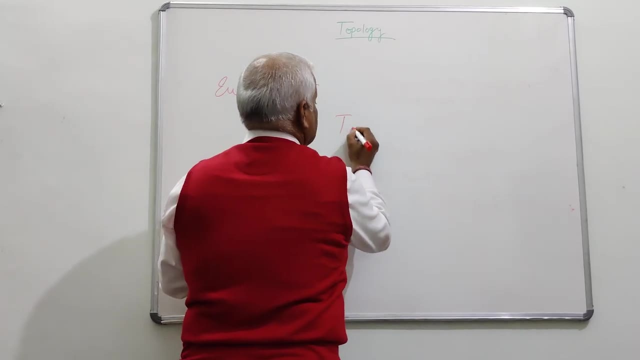 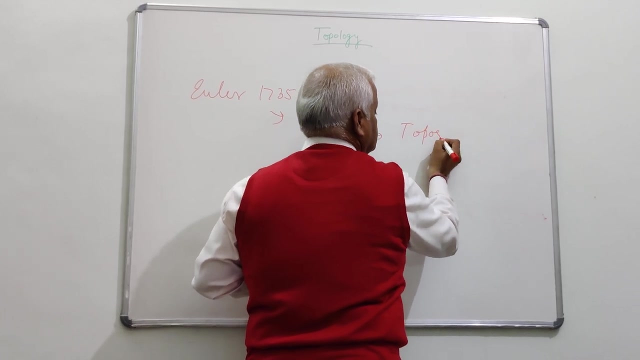 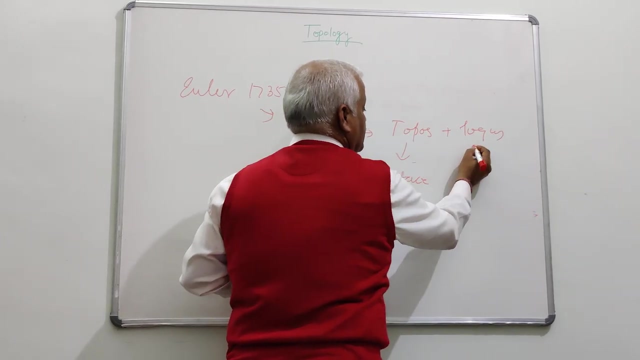 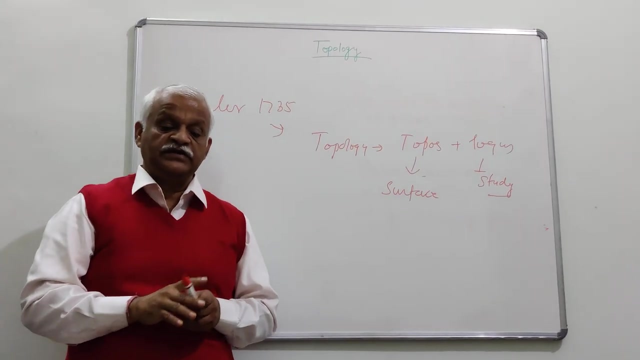 there arises the concept of topology. Actually, topology is derived from the two greek words. This topology from two greek words: topos and logos. Topos means surface and logos means study. Literally, topology means the study of surfaces. But what topology? you have to 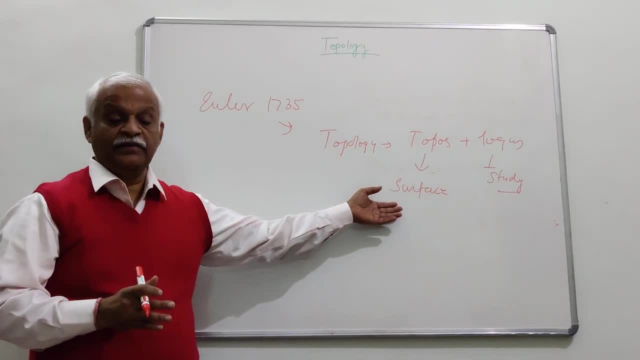 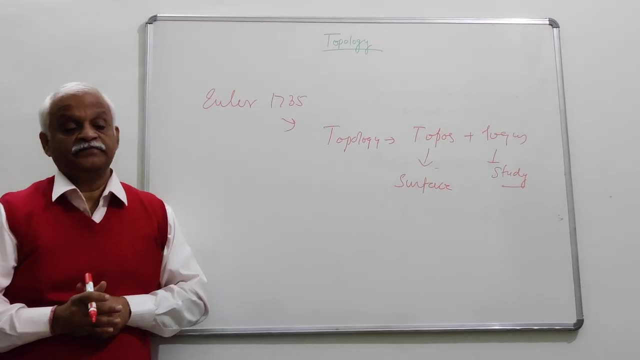 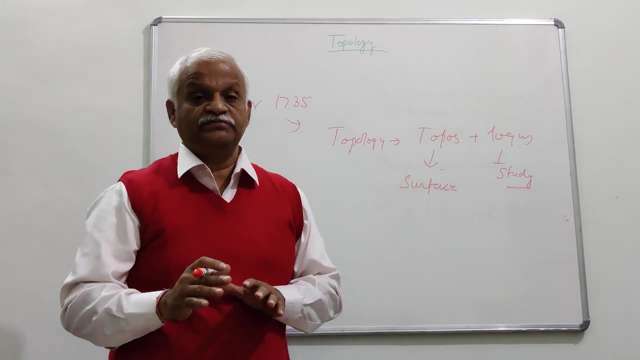 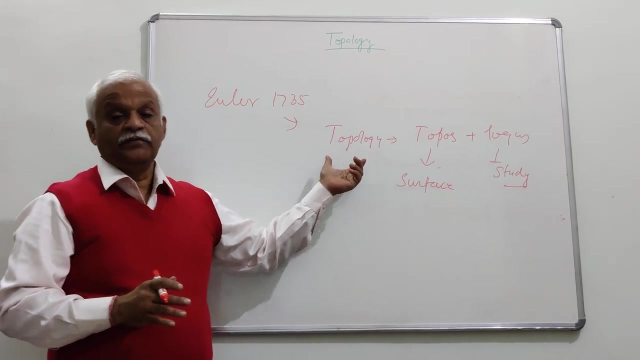 study. If you give this literal meaning, that the study of surfaces is the topology, then it is very inadequate. It is not adequate for an understanding the spirit of the subject, as you have to learn So for understanding the topology. if we want to understand the topology, then we have to. 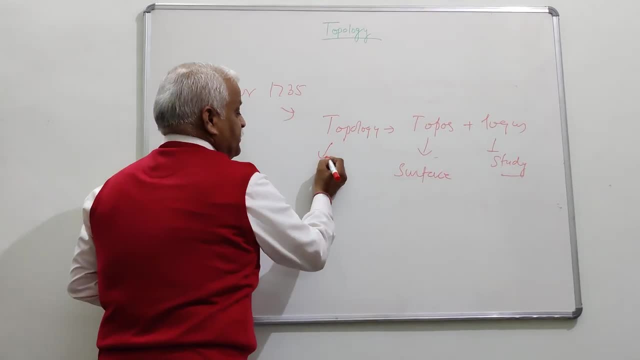 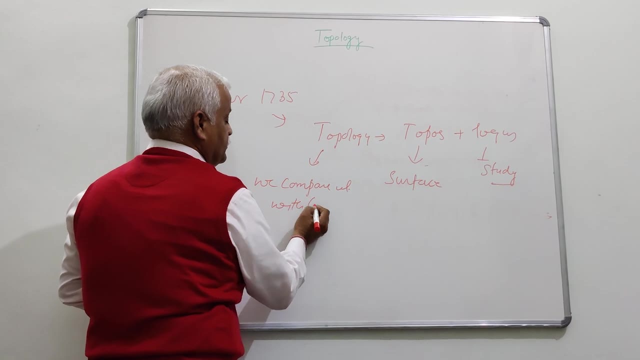 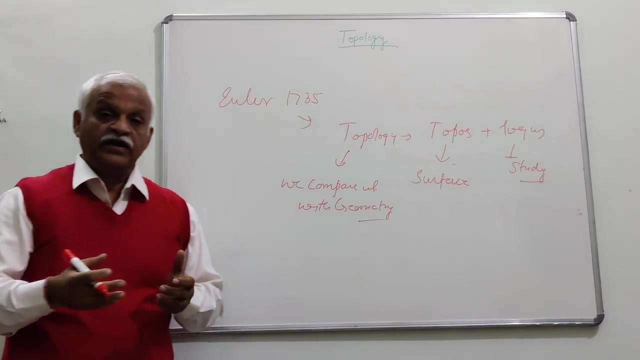 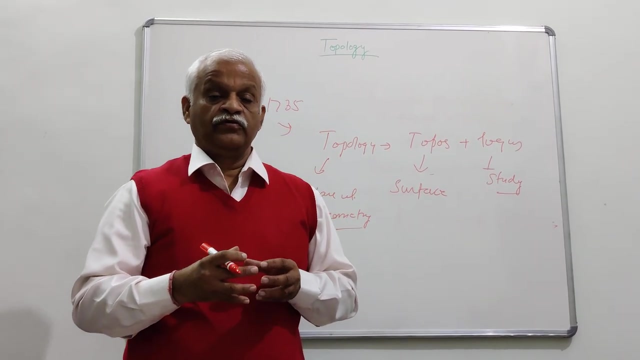 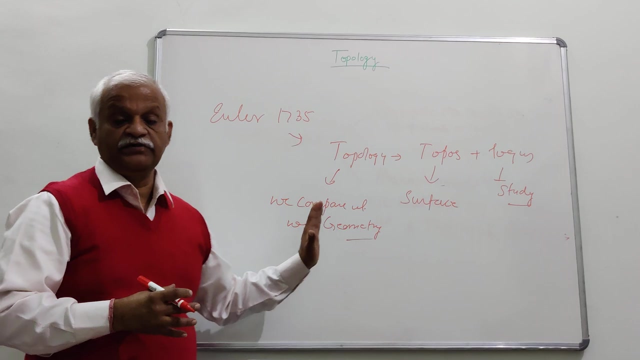 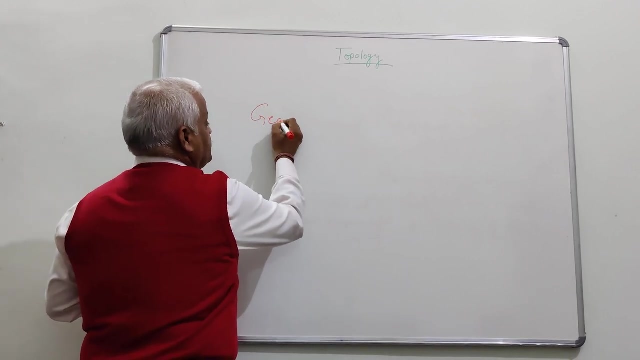 compare it first with geometry. We compare it with geometry Why? Because these two words are very similar. They are very much similar. but first we have to study about the geometry. What is geometry? Not geometry? What is geometry? You know, geometry is also a combination of 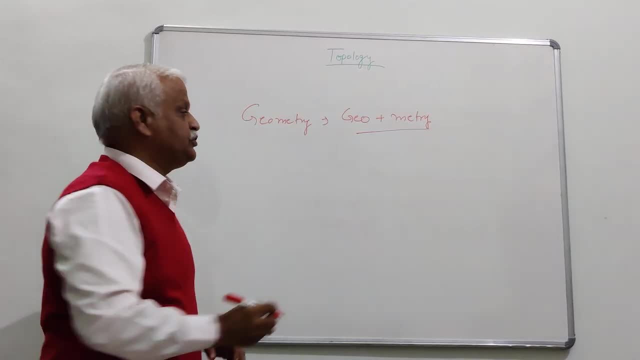 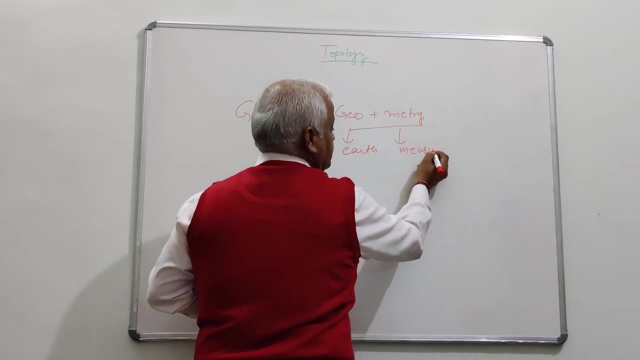 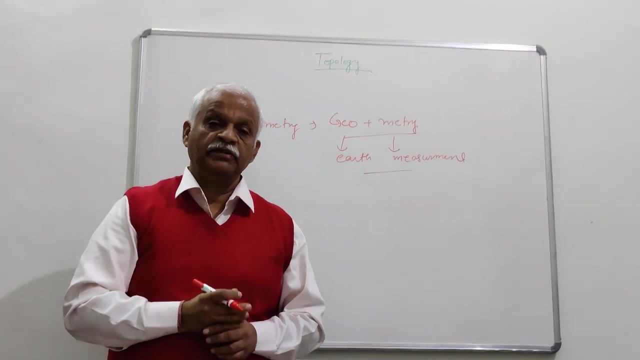 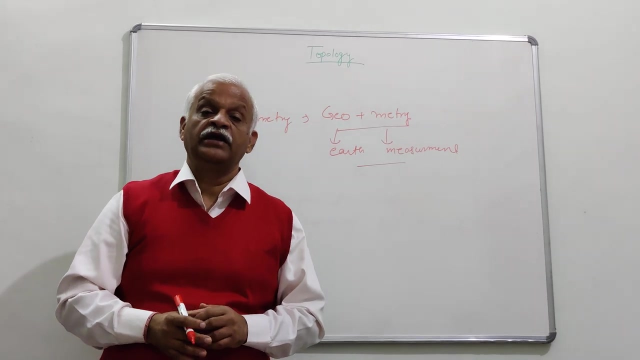 these two words: Geo plusmetry. Geo means earth and metry means measurement. So at the time of Euclid, in the time of Euclid, the use of geometry was mostly done for the measurement of earth. This was the theorem of Euclid. You must have seen the book of Euclid. You must have seen the book of Euclid. 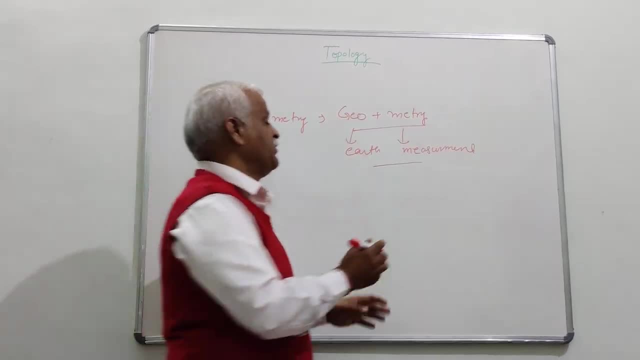 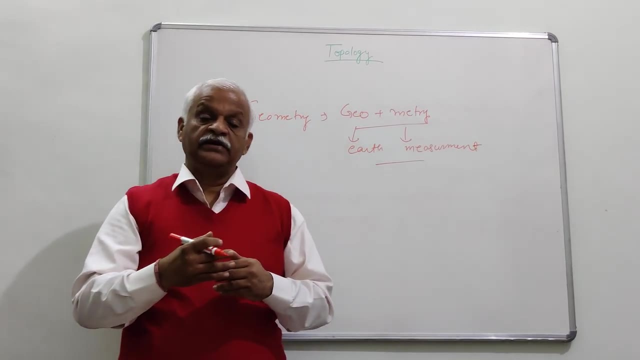 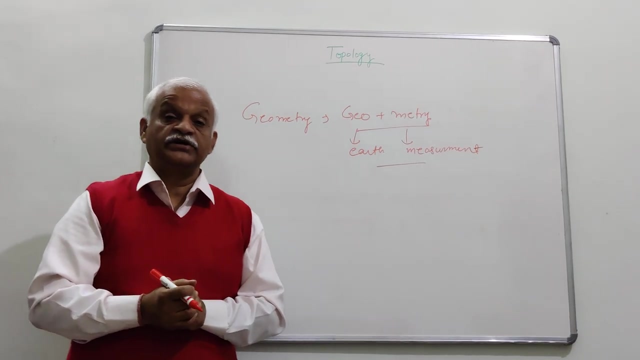 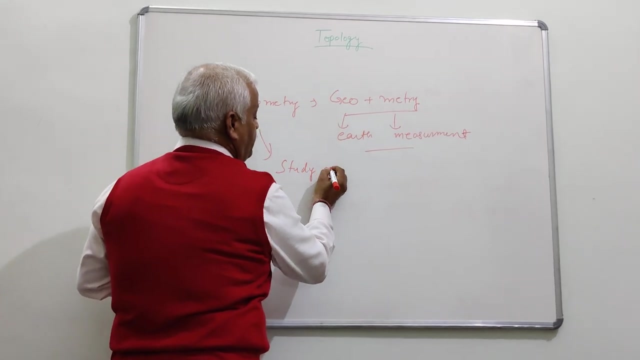 So from there, the measurement of earth was the main cause of reading geometry. But we have to study geometry according to our standard. What is geometry Here? geometry is the study of geometrical properties of object. One line definition is study of geometrical properties. 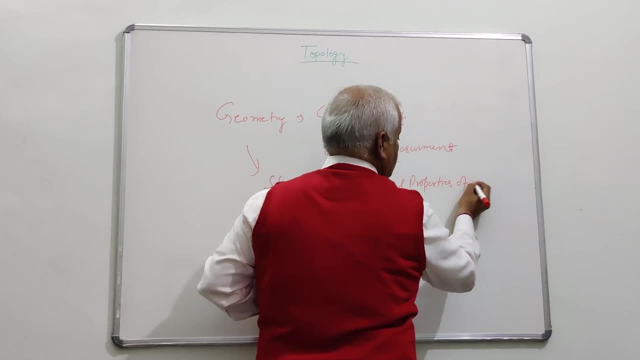 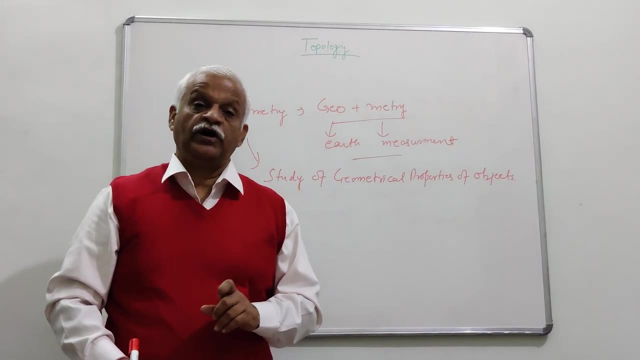 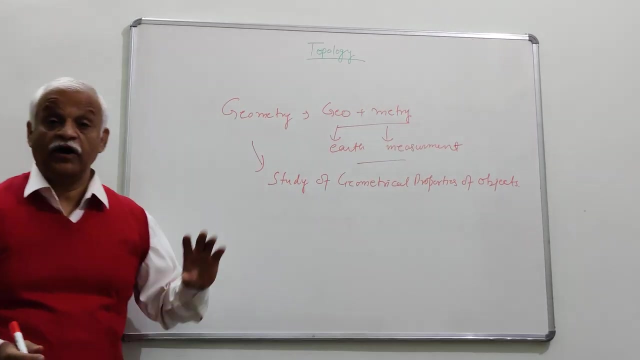 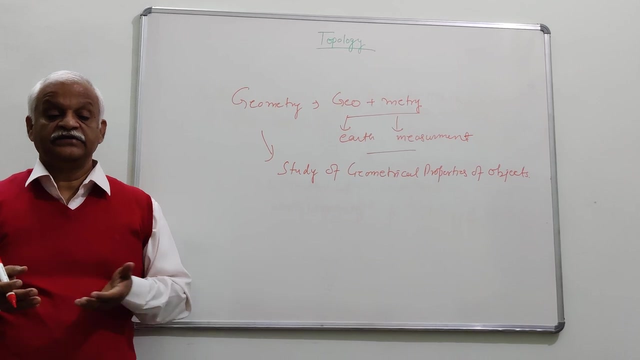 of object. when you are asked about definition of any subject, then you have to give definition of one line. that's why, in geometry you have to know study of geometrical properties of object. now, what are the objects in this? you know all about geometry. you have already studied what are lines, planes, circle, cube. they are all objects of the 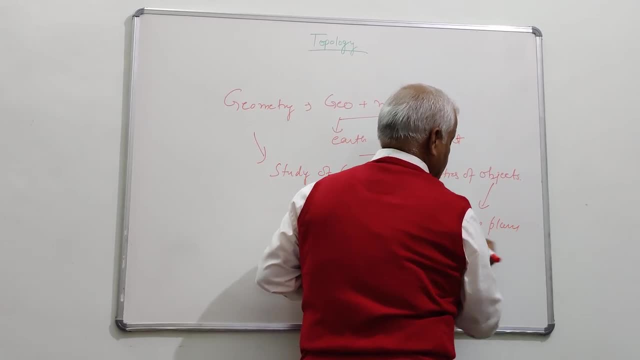 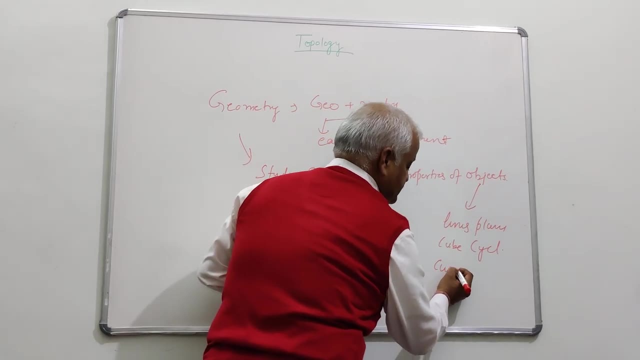 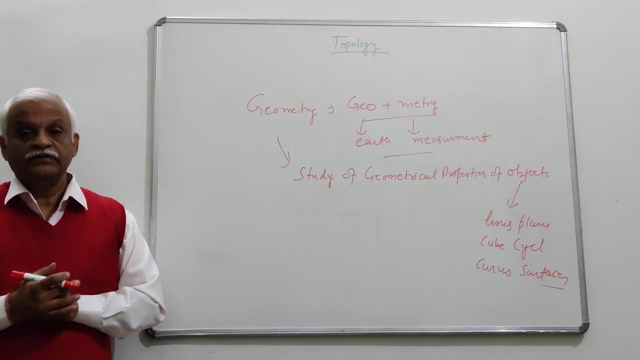 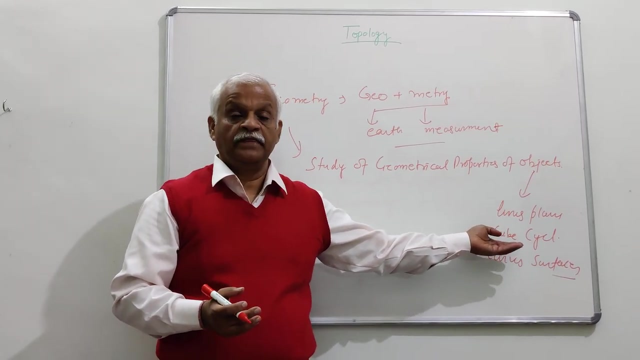 geometry lines, plane, cube, cylinder, curves, surfaces, they all are objects of the geometry and actually what these objects are. if you have to give the definition of circle, what you do? you do what these objects are. if you have to give the definition of circle, what you do, you. 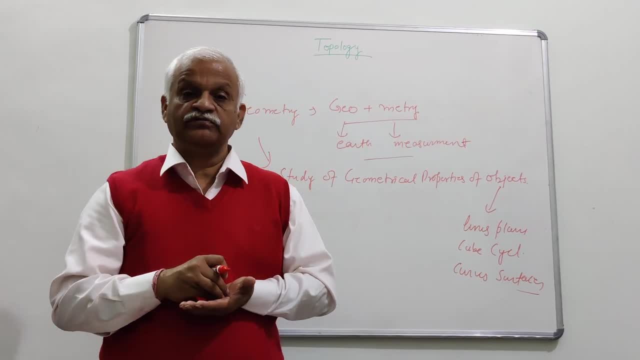 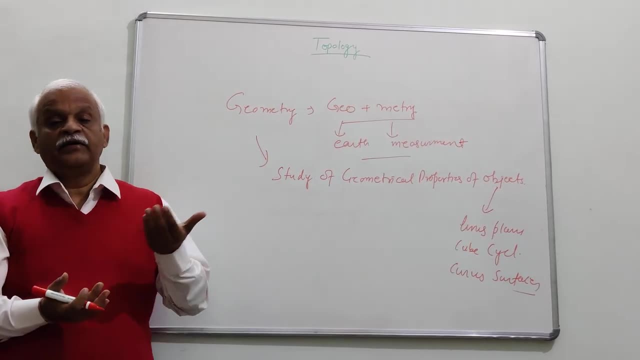 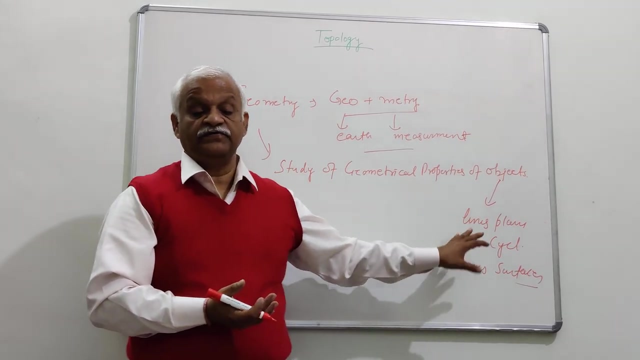 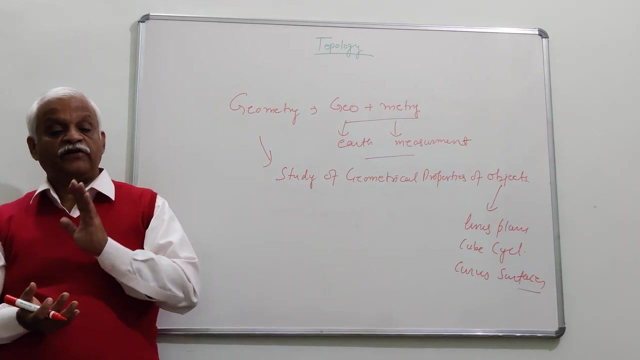 say that it is a locus of a point which moves of. that is, distance from a fixed point is always equal. you have a set of points. actually they are the mere sets. but only set is not sufficient. actually, these objects are subset of euclidean two-dimensional plane or three-dimensional surface. what are they? 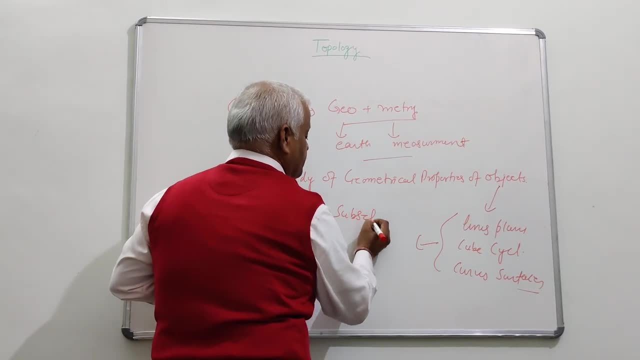 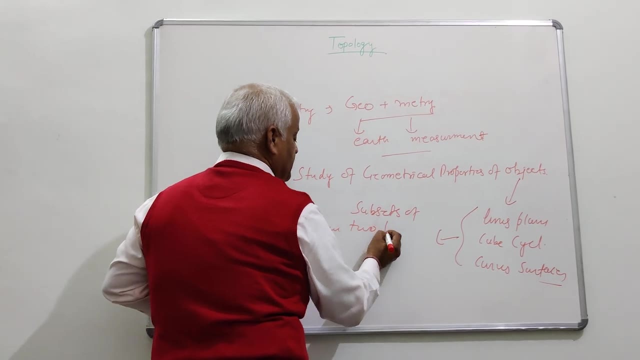 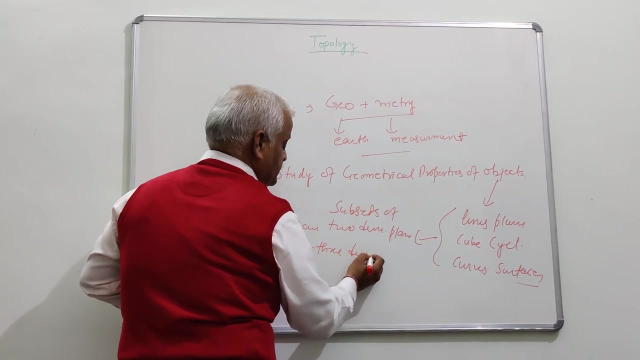 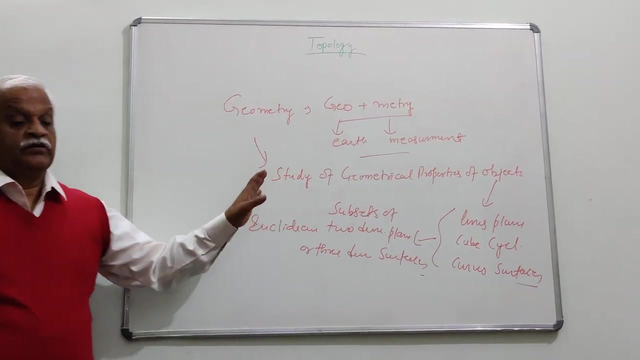 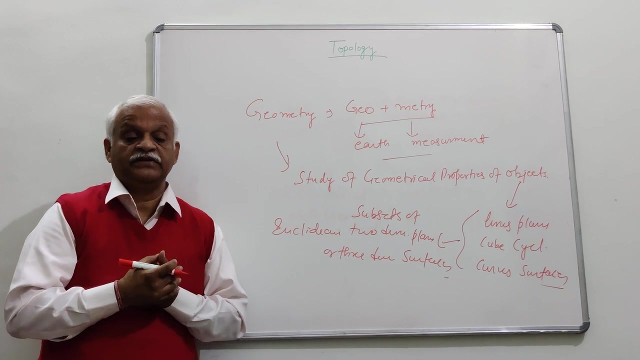 they are subsets of euclidean two-dimensional plane or three-dimensional surfaces. But they are not only the set Kewal set se kaam nahin chalega Kyun Kyunki set theory mein. aap kya padte hai? 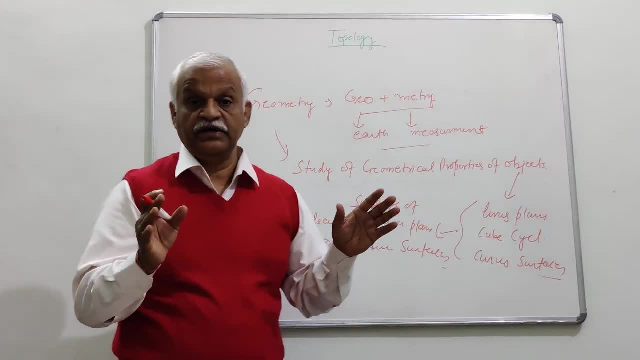 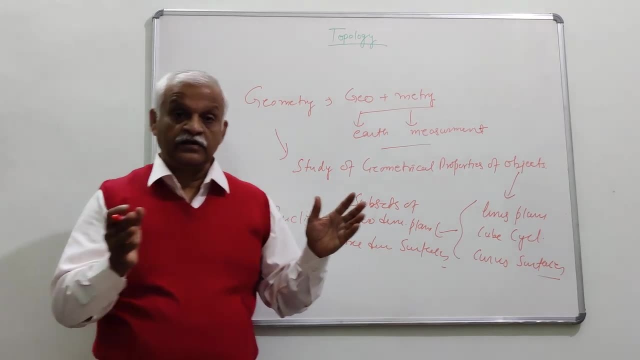 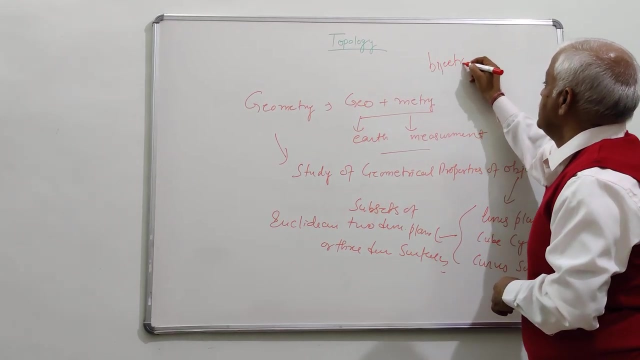 Ki there exists a bijection. Bijection means one one on two mapping. Aur jab do chijon ke beech mein bijection hoga. Bijection means: What is the meaning of bijection? Bijection is one one on two mapping. 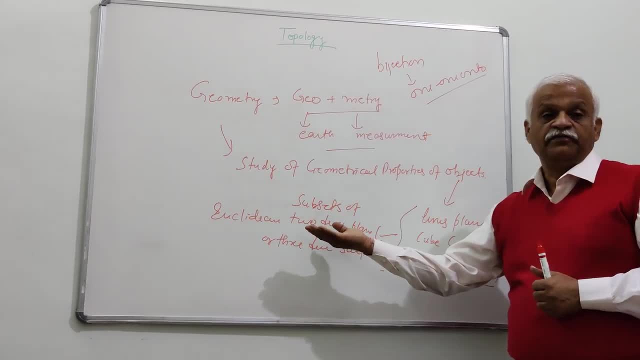 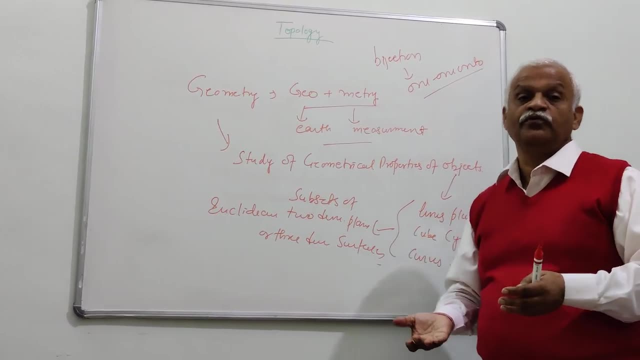 But if in sets of points ke beech mein lines aur cylinder ke beech mein, agar ye one one on two mapping exist karti hai, iska matlab, ki dono mein koi fark hai hi nahin, Aur agar dono mein koi fark nahin hai. 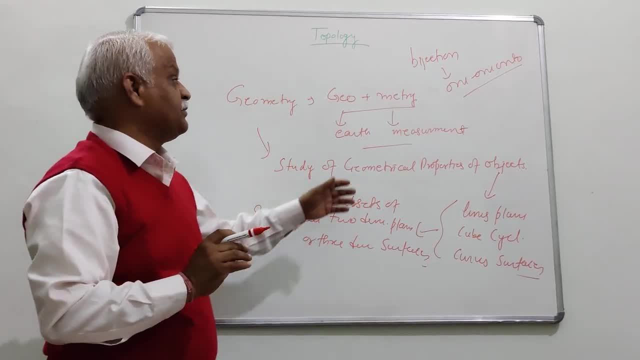 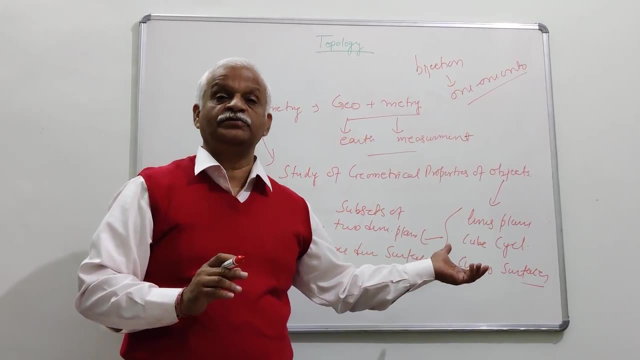 to iska matlab. kya hua? Iska matlab hua ki object C aur ye objects ka same huna jo hai. this is the disaster for the geometer, Because in geometry you see the objects, Agar aapko lines aur cylinder. 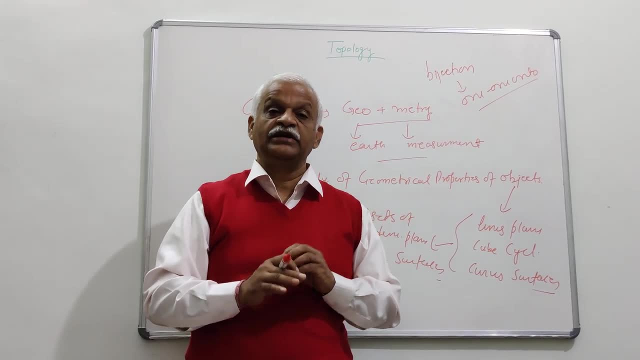 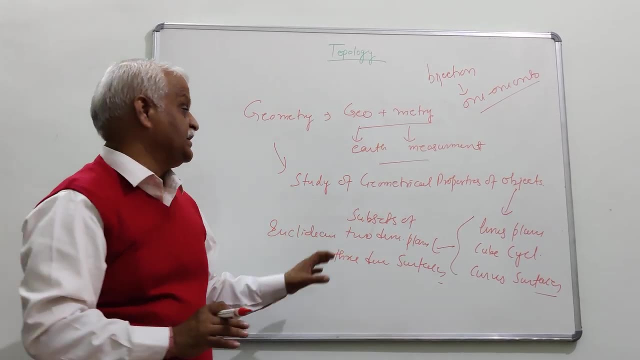 ek yasi dikhayi de rahi hai Iska matlab, jo geometry ki kalpana thi wahi maha nast ho gayi. So it means there is some additional thing which is involved in this geometry, And this is the geometrical properties. 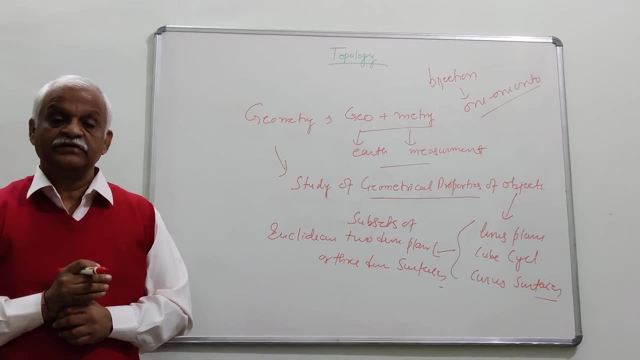 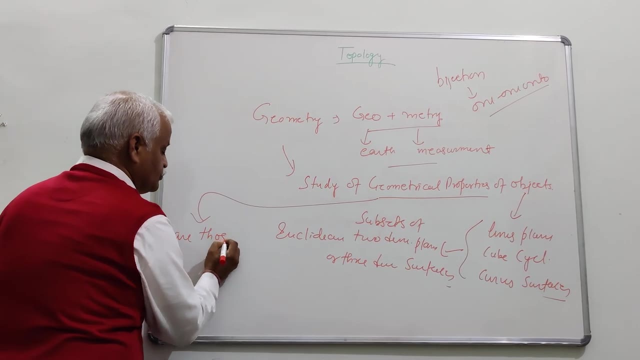 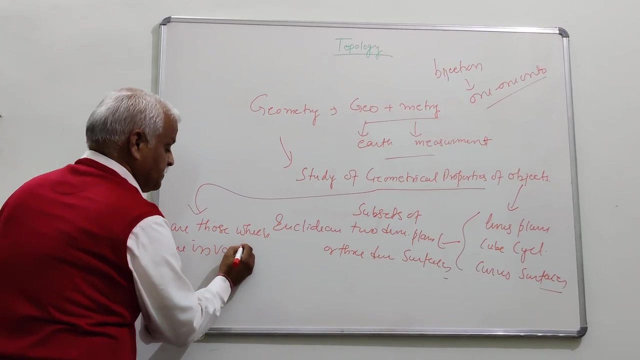 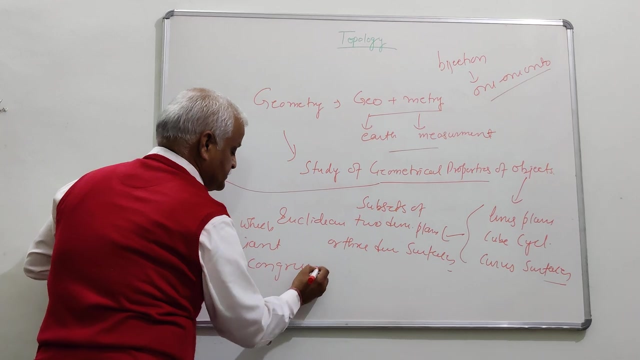 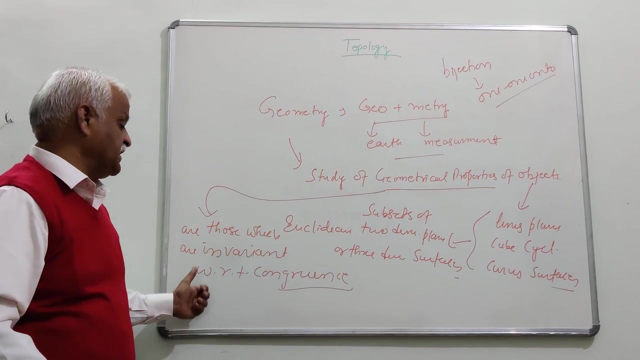 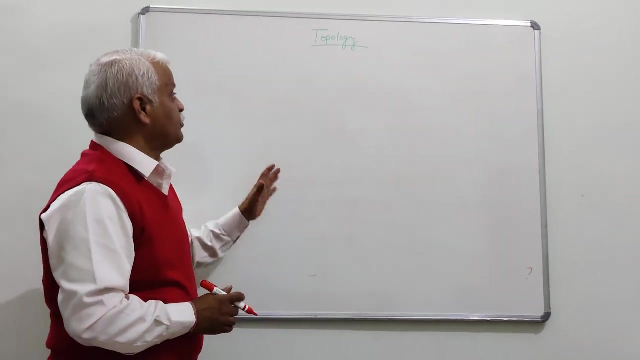 What are the geometrical properties? Geometrical properties are those which are invariant with respect to congruence. And now look at this: Which are invariant with respect to congruence, And what is congruence? So the geometrical objects are not merely a set. 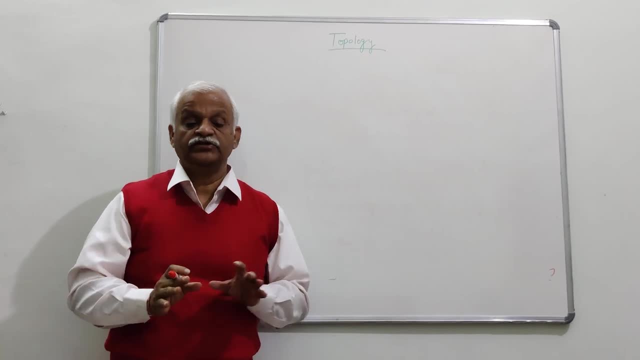 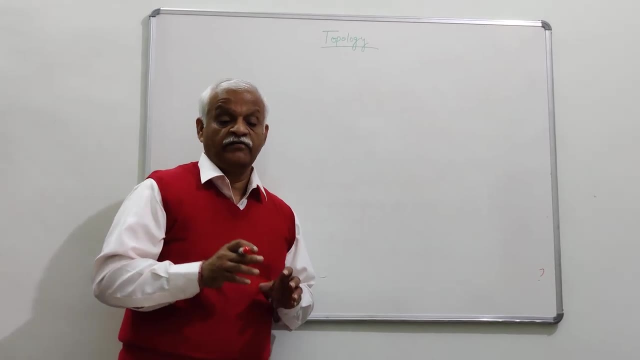 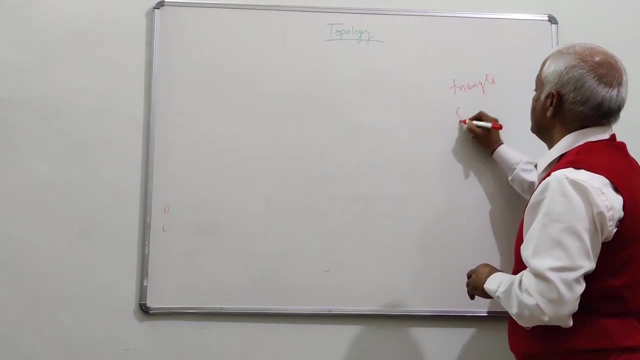 Because if they are only set, then this is the disaster for the geometer Means. it must have some additional structure. And for what? For what which can distinguish between triangle and square, How these two are different Means. you must have the additional structure. 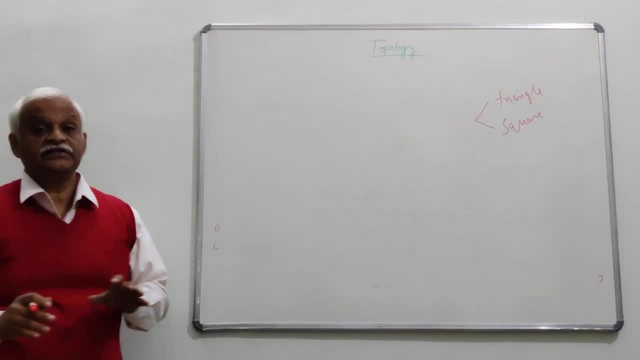 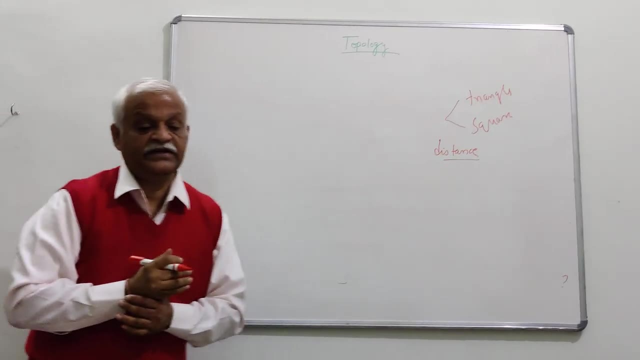 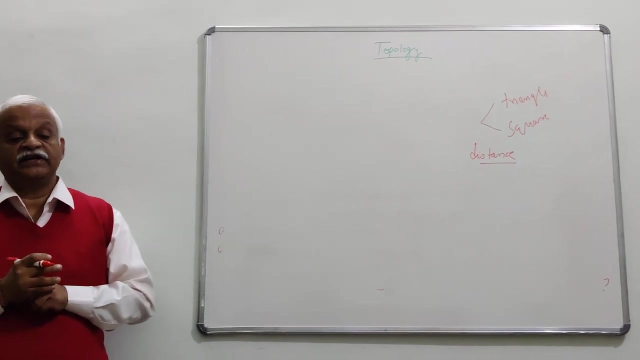 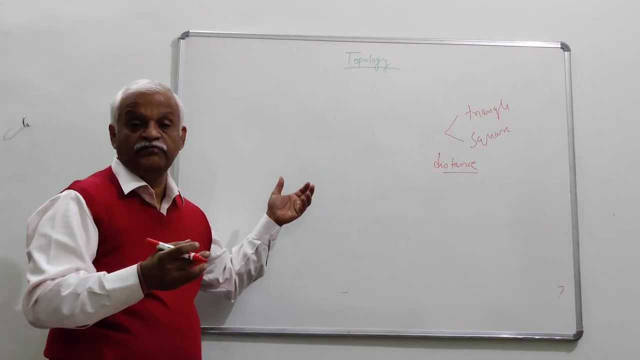 And you know what is that additional structure? That is distance. That is distance And there are so many geometry. We deal with things like volume, curvature, etc. Which are the geometrical properties, And now we define the geometrical properties. Geometrical properties: I have already told. 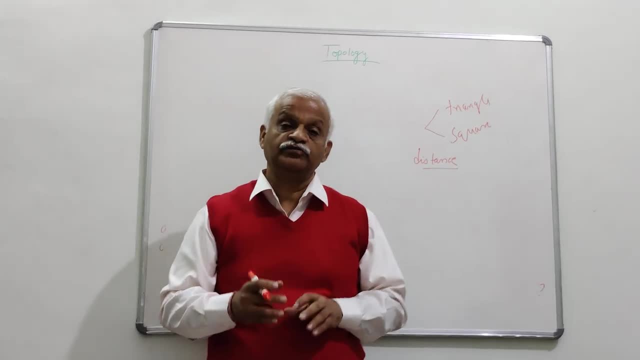 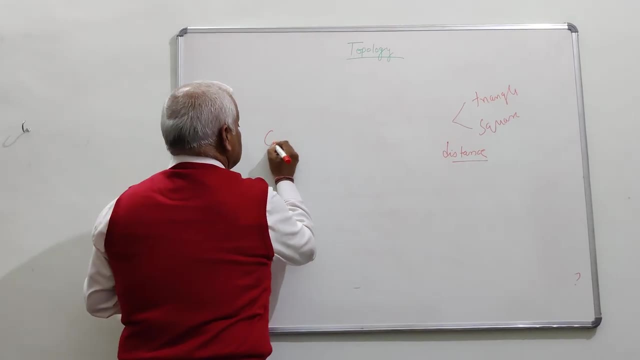 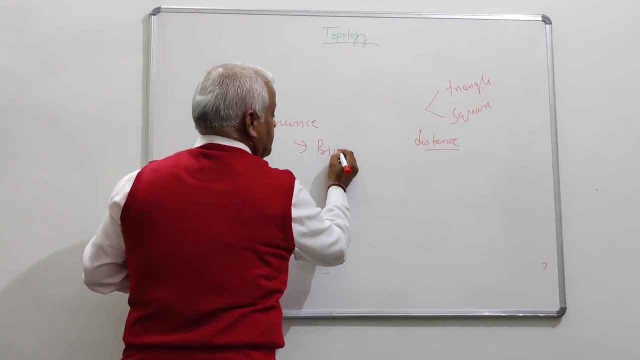 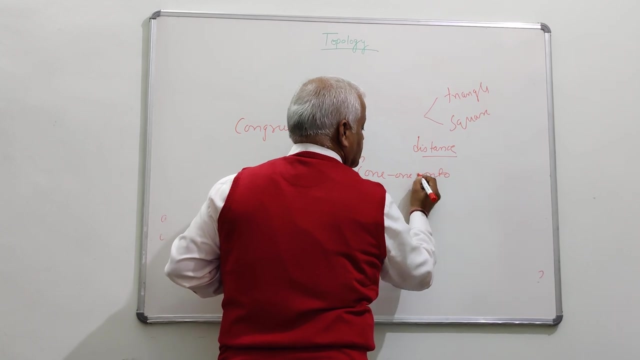 What are the geometrical properties? Geometrical properties are those which are invariant with respect to congruence, And congruence has two things: One is bijection One-one onto mapping And second thing, it preserves the distance. What is distance? 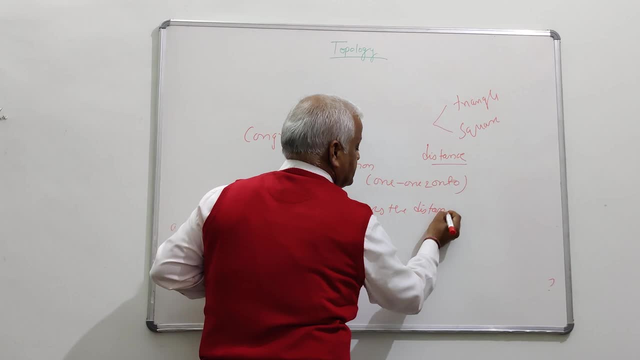 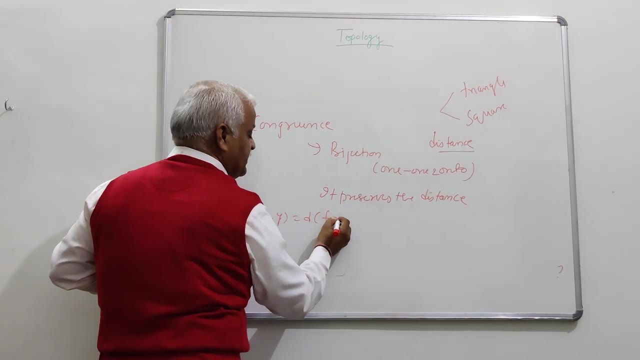 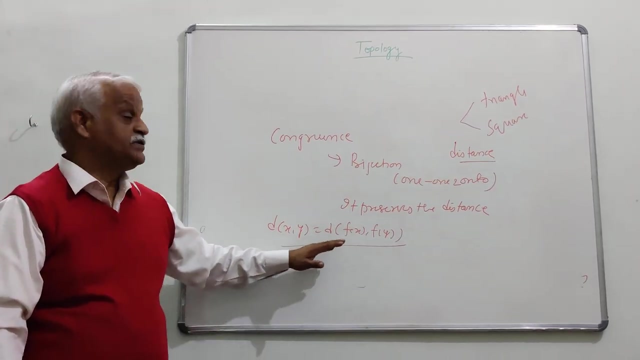 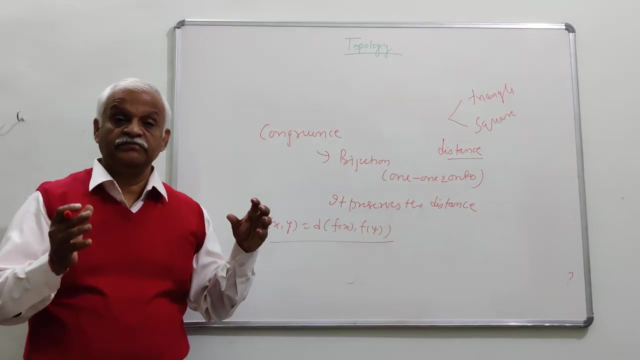 Preserves the distance means d x- y is equal to d of f x f y. This is the initial thing Which we have in congruence Means. it is not only the set Set with bijection Means if two sets are congruent. 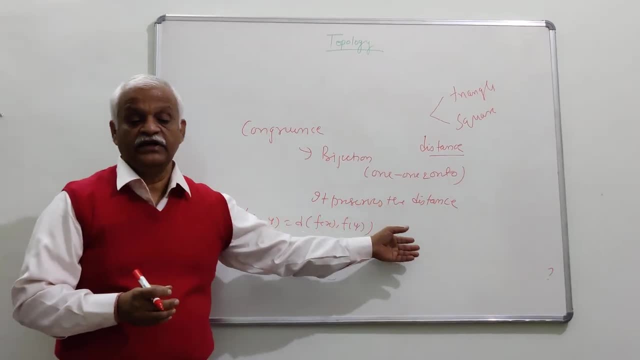 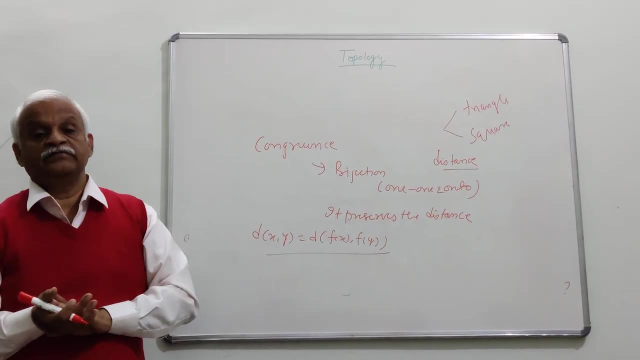 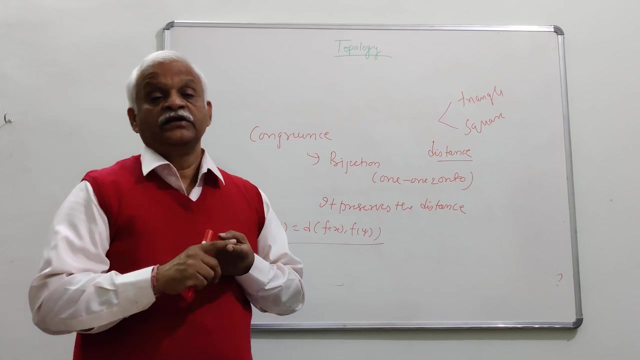 They have the bijection As well as they preserve the distance, Because preserving of distance is very much necessary for this geometry. So in geometry, in one line definition You have, geometry is the study of geometrical properties of object. If you tell the definition of one sentence, 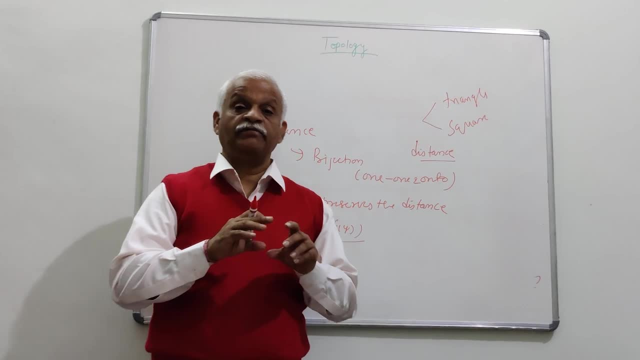 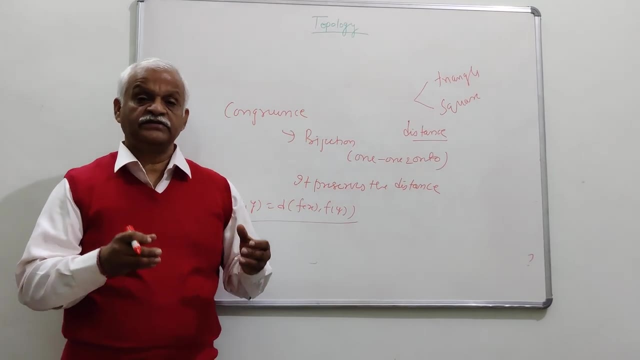 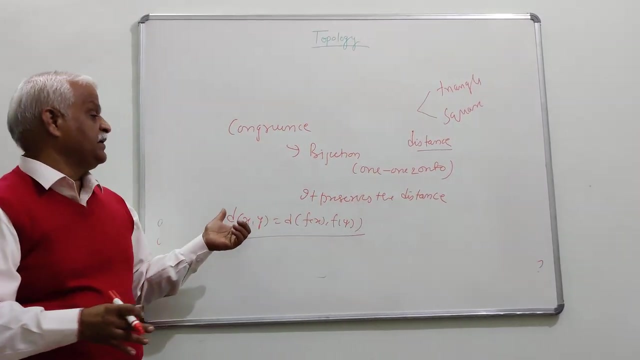 Then you are a little bit stuck. Why? Because when you ask what is the object, There are the lines, Circles, Cubes, Surfaces, Curves, All that. So what are the geometrical properties? Did you tell the geometrical properties in one line? 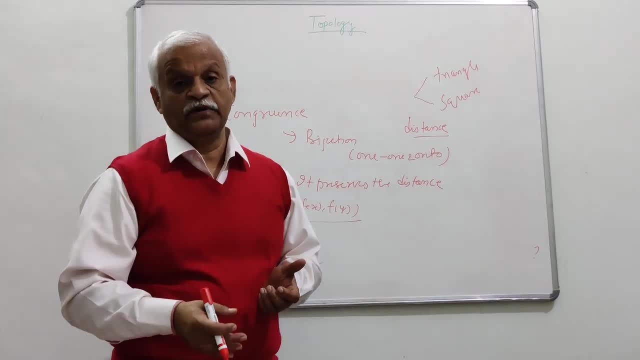 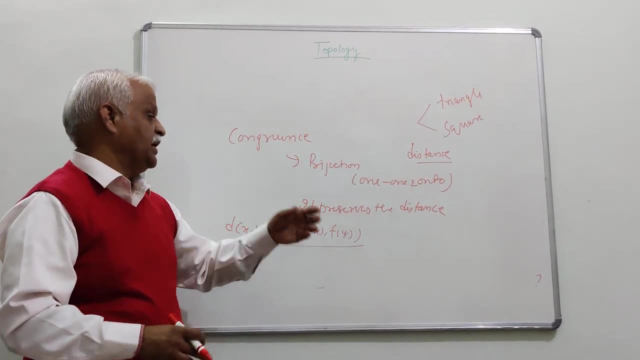 What Geometrical properties are those properties which are invariant with respect to congruence? Now you ask: what is congruence? Congruence means bijection, And it preserves the distance. So what is there in congruency? These two things. 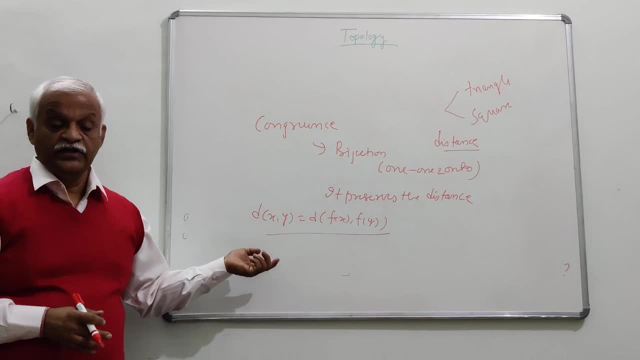 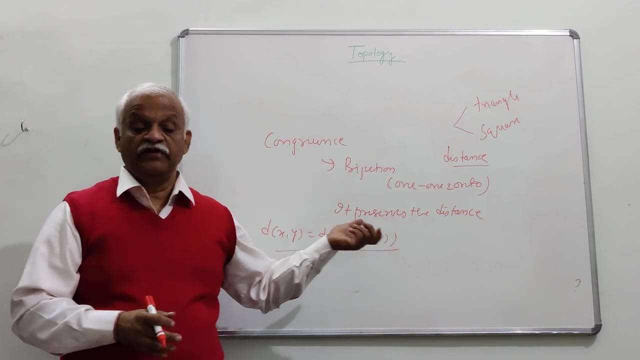 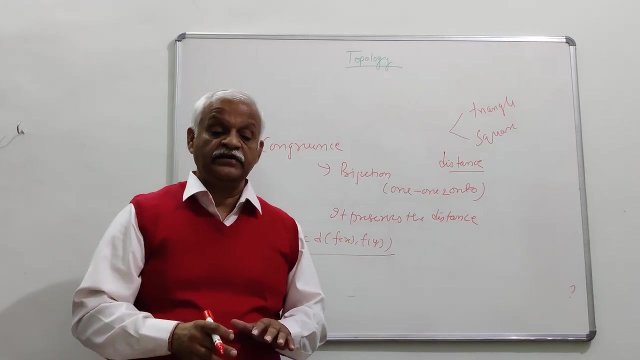 Whenever an object has the property, Then it preserves the distance, So does every object congruent to it. Invariant means this. Invariant under congruence means Whenever an object has that property, So does every object congruent to it. 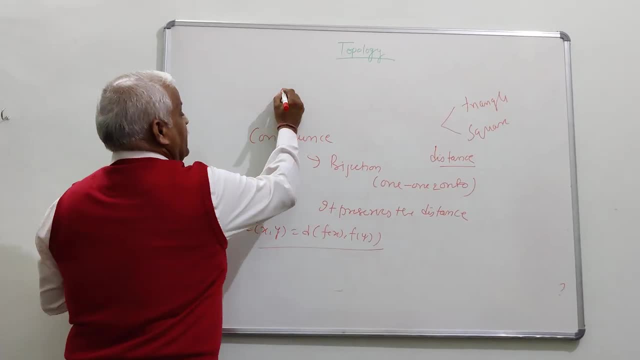 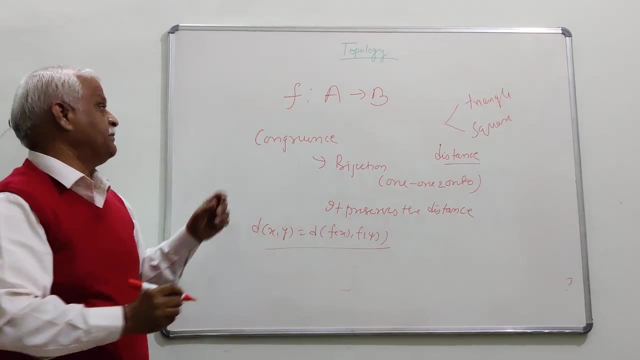 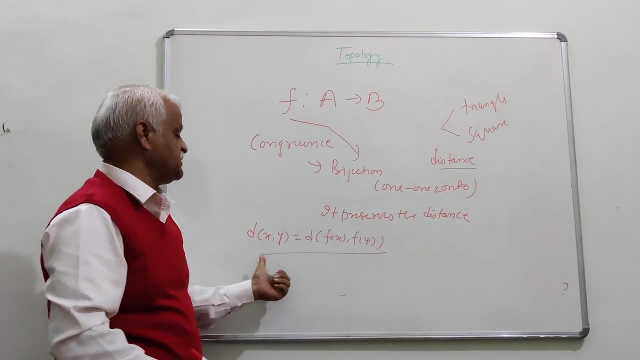 So if F is the congruence between this A and B Means F, A to B is the bijection, F is bijection Means one one onto mapping And it preserves the distance D of XY is equal to DFX and FY. 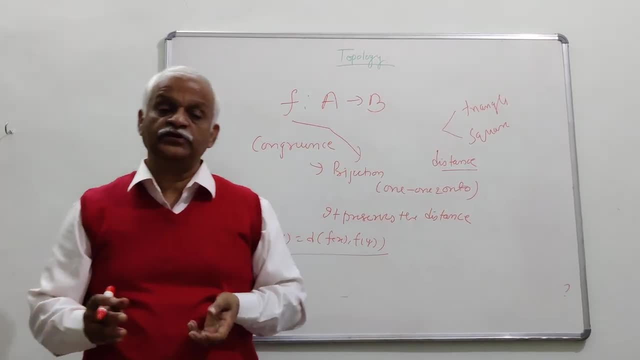 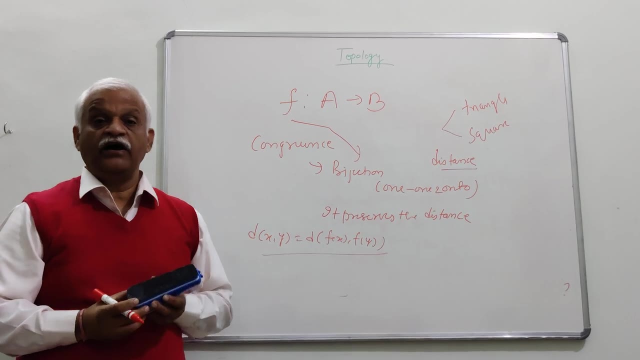 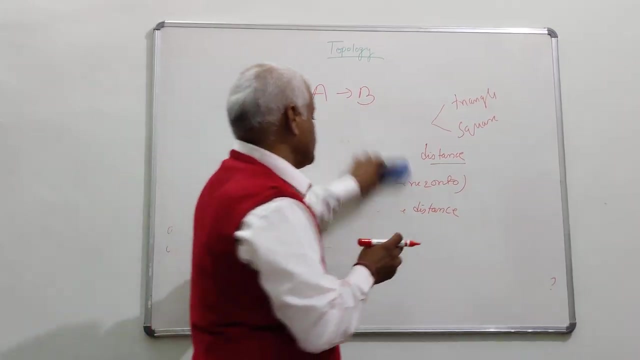 Same definition you have for set theory also. What is set theory? Because set is involved in this. In set theory, Set theory is the study of set theoretic properties of object. What is set theory? Because set is involved in all these. 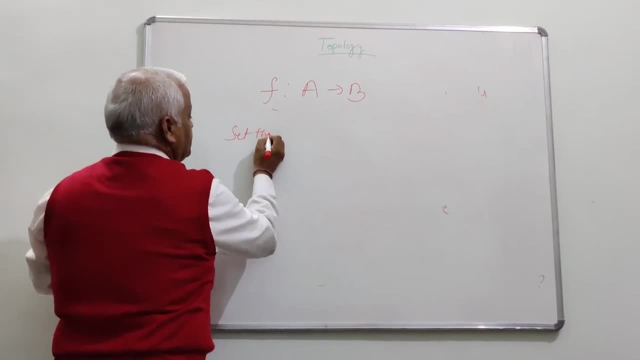 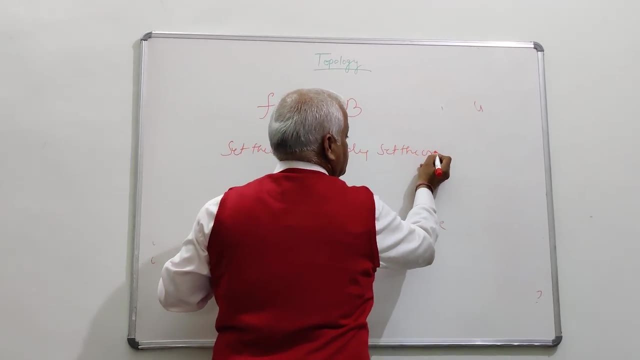 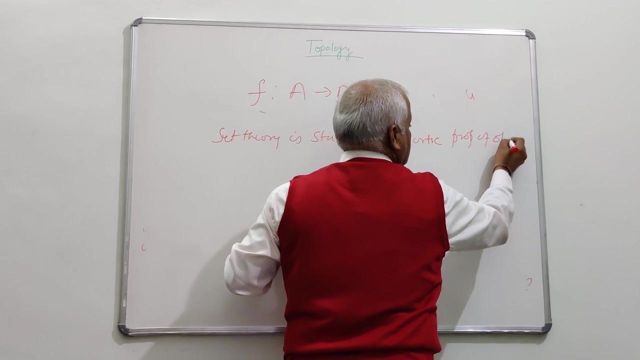 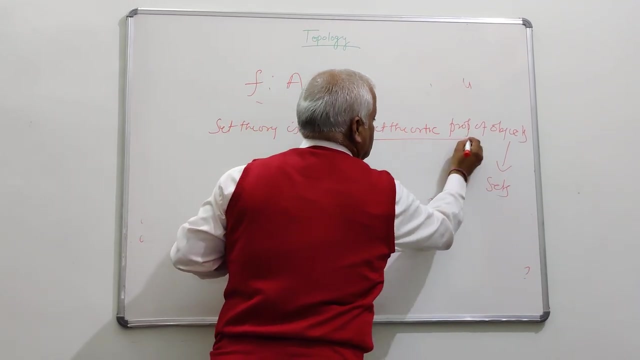 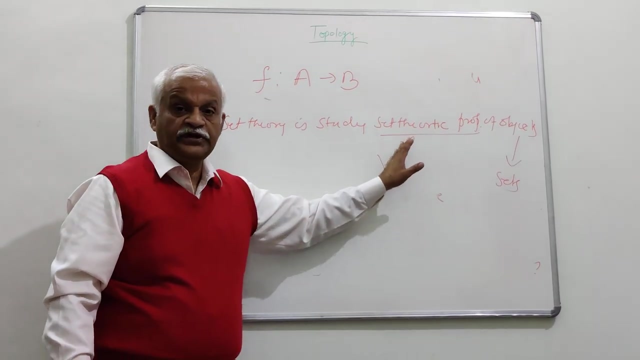 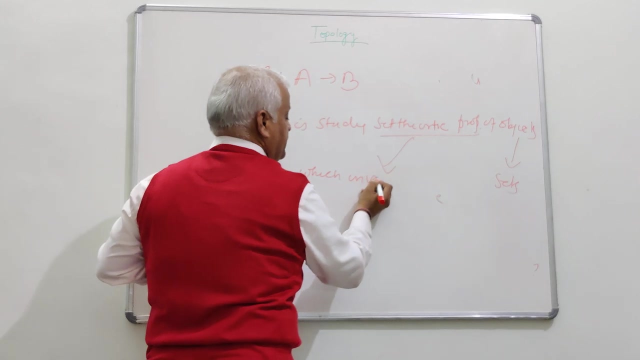 Set theory is the study of set theoretic properties of objects. Now, here the objects are different, Objects are sets. What are the set theoretic properties? What are set theoretic properties? Same definition: Set theoretic properties are those properties Which are invariant. 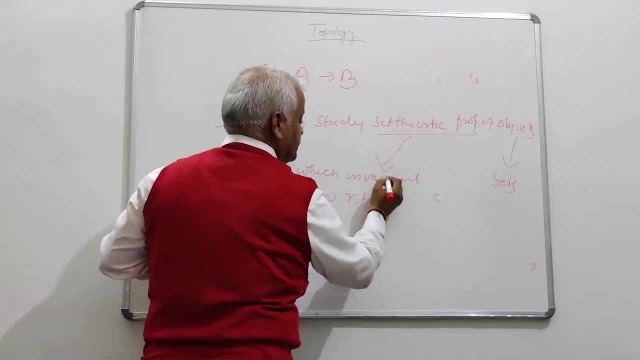 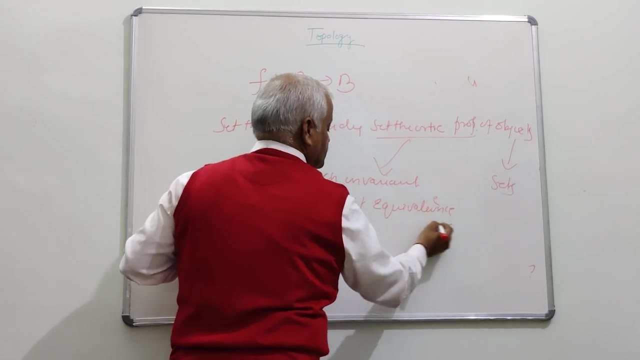 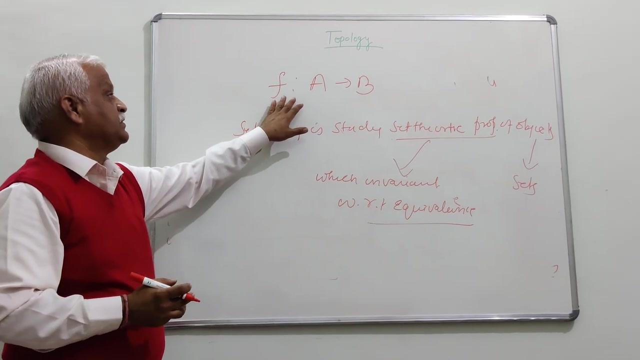 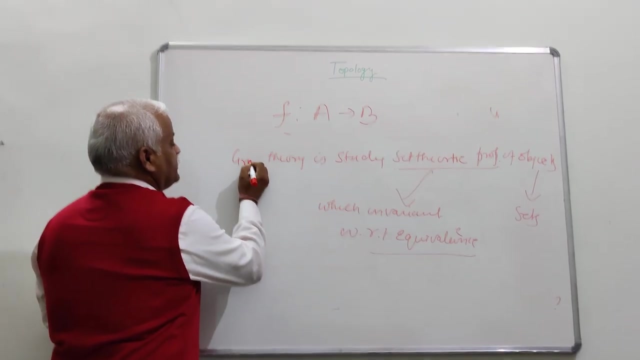 With respect to Equivalence, With respect to equivalence. Right Now look at the group theory. also In group theory, The same definition: Group theory is the study of Group theoretic properties of object. Group theoretic properties of objects. 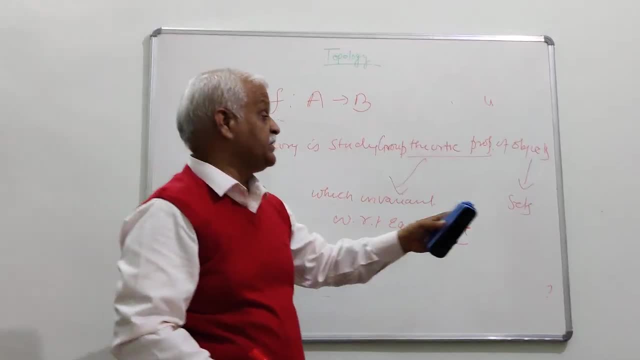 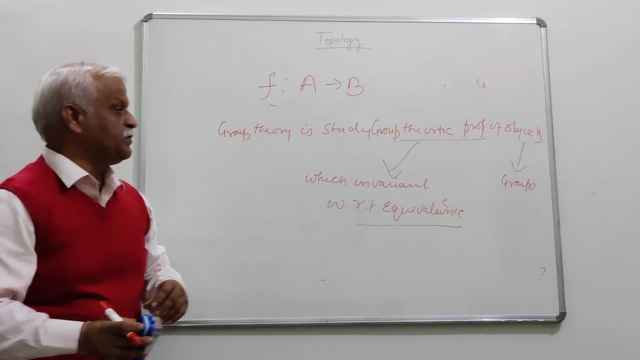 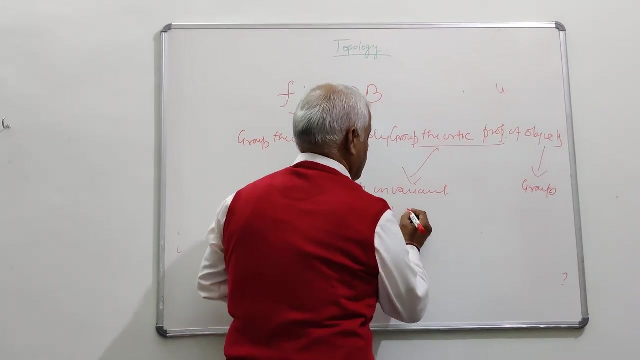 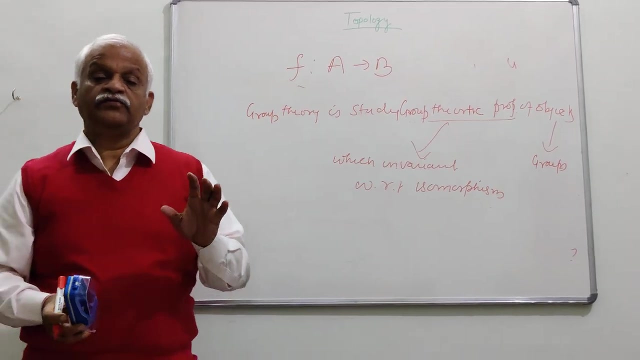 Here the objects are the group. And what are the group? theoretic properties Which are invariant with respect to isomarkets. Isomarkets are the set of the group. just i am telling that if you give the definition of anything, you have to give the definition in. 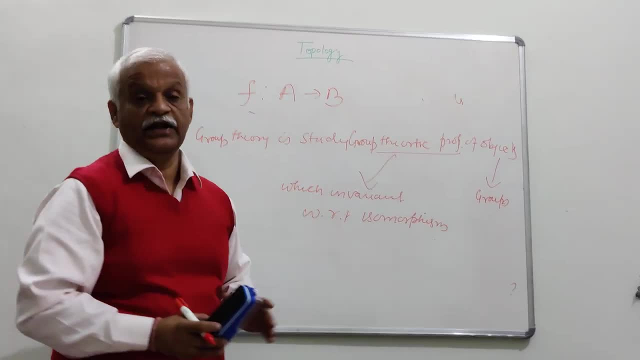 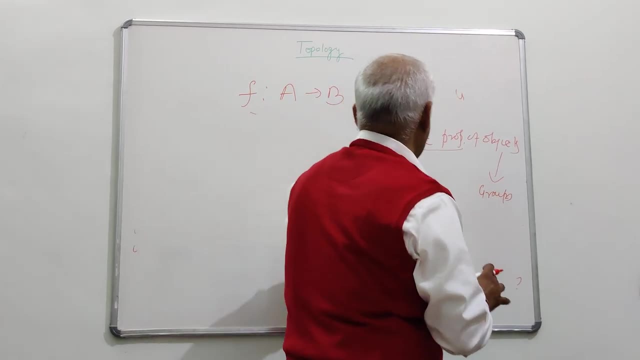 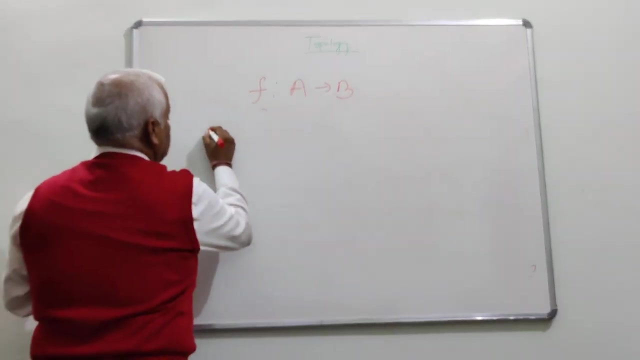 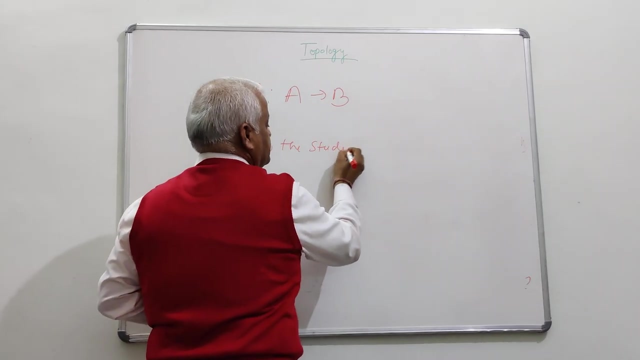 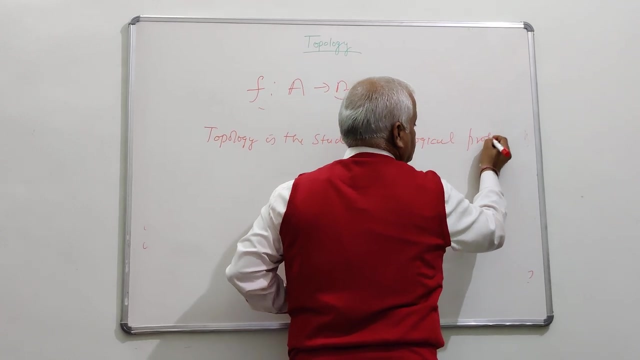 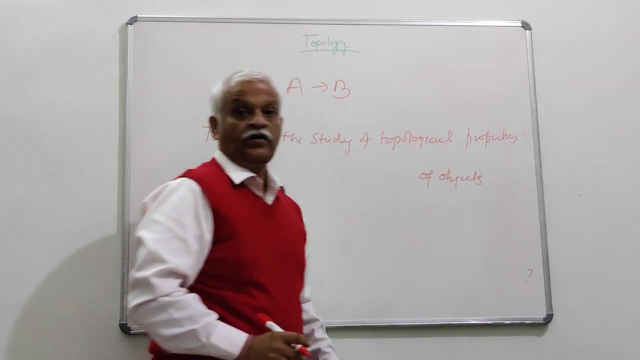 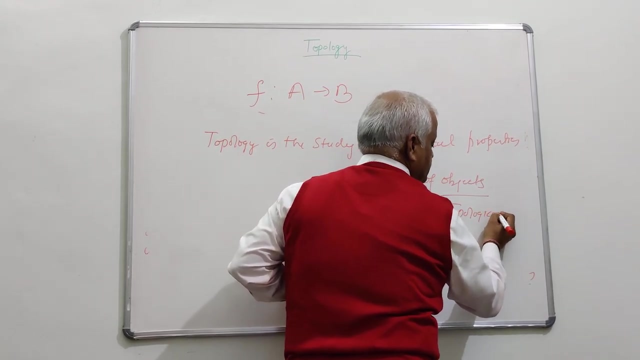 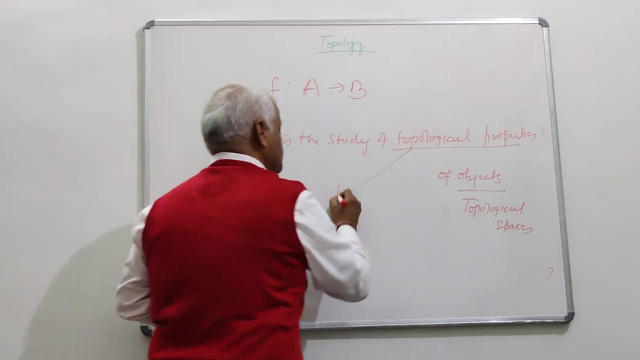 one line. now we come to our subject. what topology is right? in the same manner, we have to give the definition of the topology. what topology is? topology is the study of topological properties of objects. now, here, the objects are topological species, objects are topological species. and what are the topological property? the same question: what are?